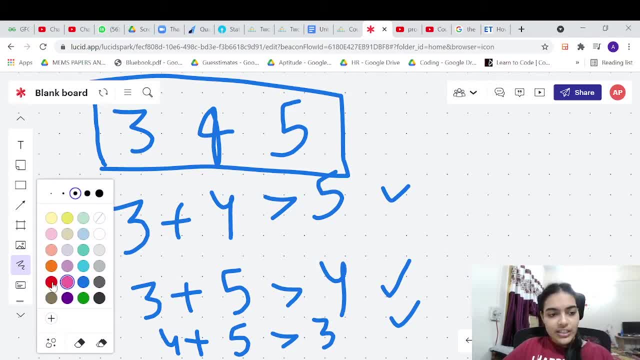 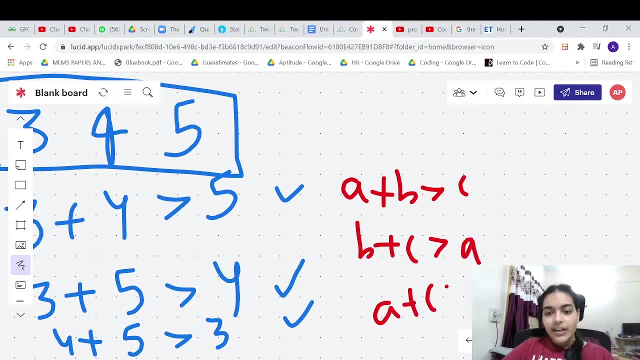 using three numbers. you just need to satisfy three conditions. and what are those three conditions? a plus b is greater than c. b plus c is greater than a. a plus c is greater than b, right, Where a, b, c represents the side of the triangles. If you satisfy these three conditions, you will be. 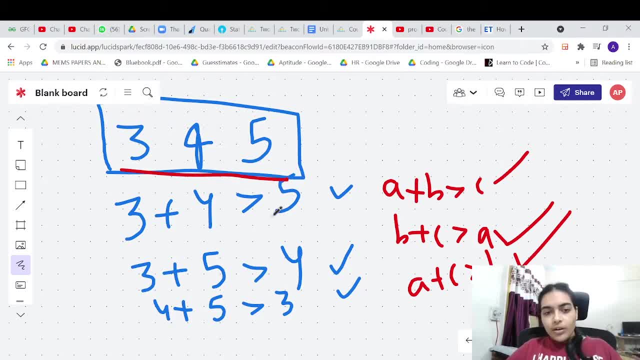 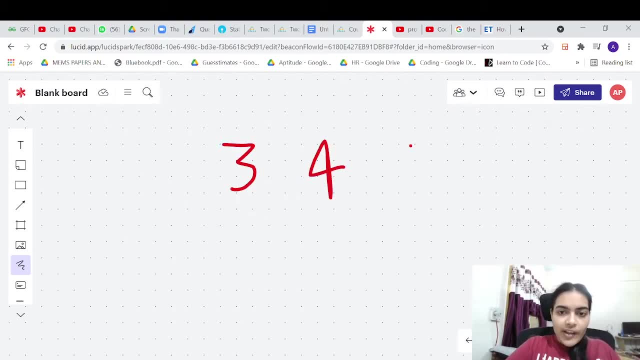 able to form a triangle using three numbers. okay, Now let's try to take some example where we can not form a triangle. Let's see what is the problem. Suppose you have three numbers: 3,, 4, 8.. 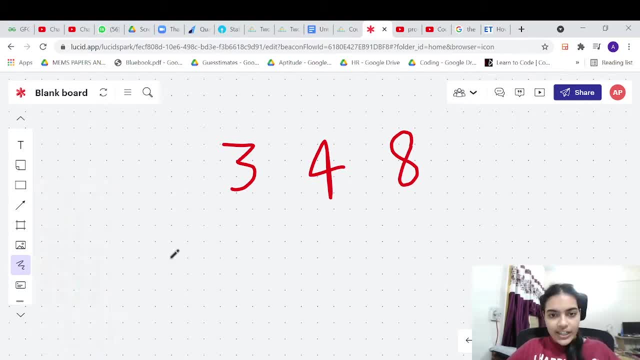 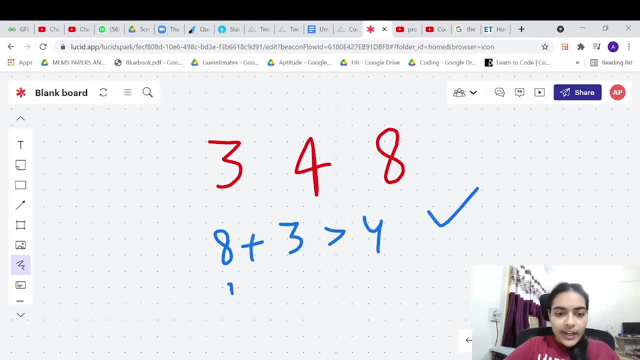 Can you form a triangle using these three numbers? Okay, let's try to check the conditions one by one. 8 plus 3 is greater than 4.. This condition is satisfied, right. 11 is greater than 4.. 8 plus 4. 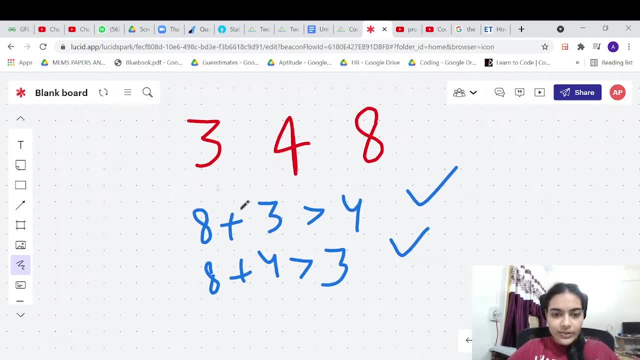 is greater than 3.. 12 is greater than 3.. This condition is also satisfied. But when you come to this condition- 3 plus 4 greater than 8, this condition is not getting satisfied, right? 7 is greater than 8 is not getting satisfied, okay. 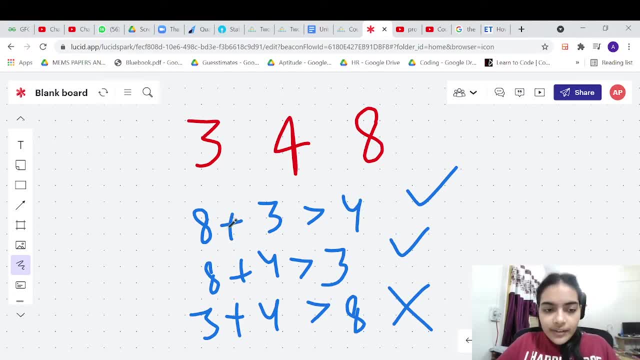 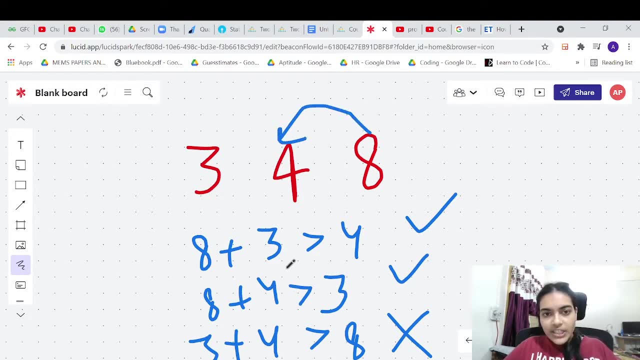 This is false. Now try to observe one thing here. right, This condition, these two conditions, were not failing. 8 plus 3 and 8 plus 4 was not failing. Which condition is failing? This condition is failing. okay, Now is there some special reason why these two conditions were? 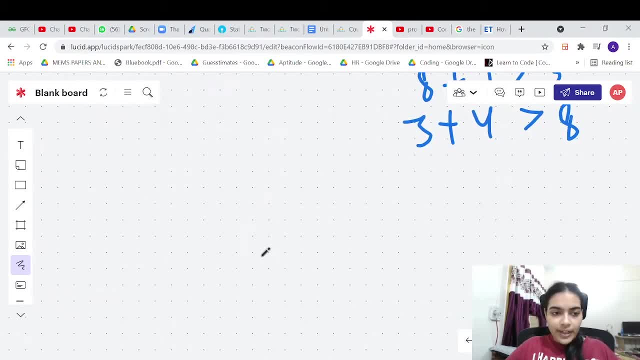 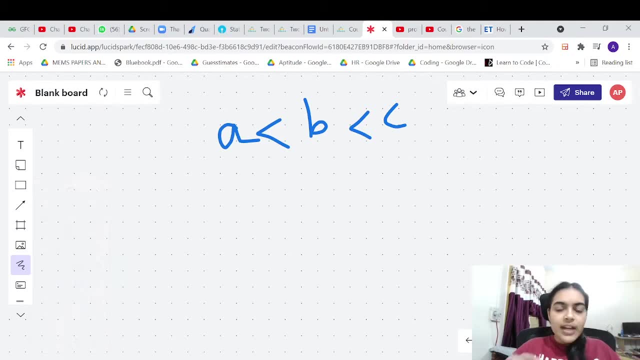 passing. Let's try to understand it even better. okay, Let's say you have three numbers right- a, b, c, where a is less than b and b is less than c. okay, Let's take ascending order simply to. 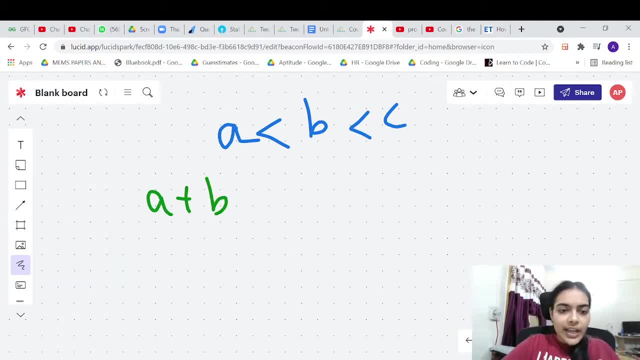 understand the logic right now. So we have to check three conditions right: a plus b greater than c, b plus a greater than c. and sorry, these two conditions are same. Let me write them again: a plus b greater than c, a plus c greater than b and b plus c greater than a. right, You have to. 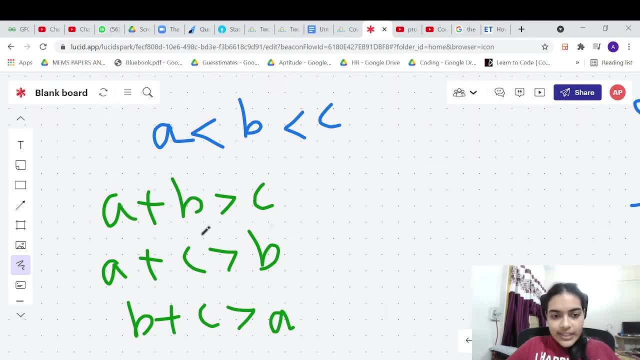 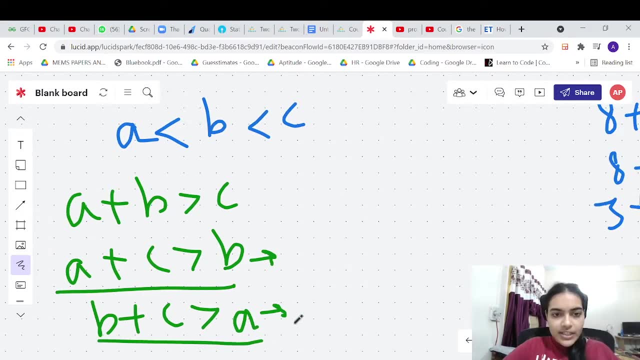 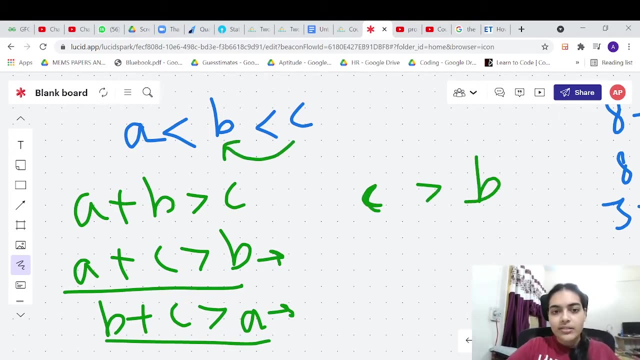 check these three conditions. Now let's try to analyze these two conditions. okay, So these two conditions are very special. Why? Because, see you know one thing: c is greater than b. right, c is greater than b because they are in ascending. 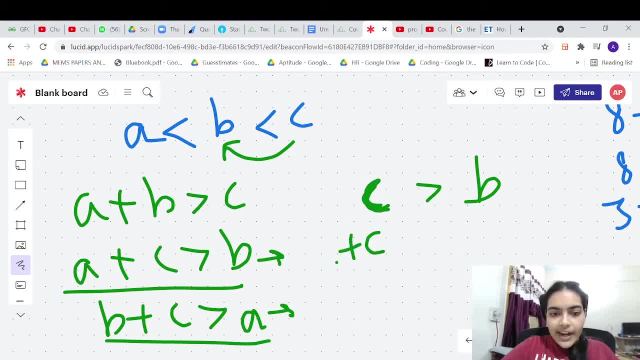 order. Since c is greater than b, let me add a to both sides. okay, c plus a will be greater than b plus a, or c plus a will be greater than b plus a. right, c plus a is greater than b plus a. That. 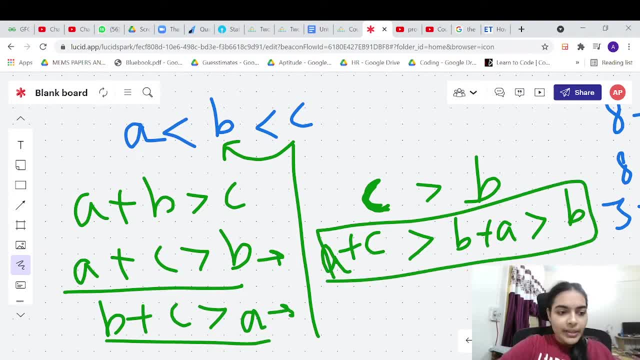 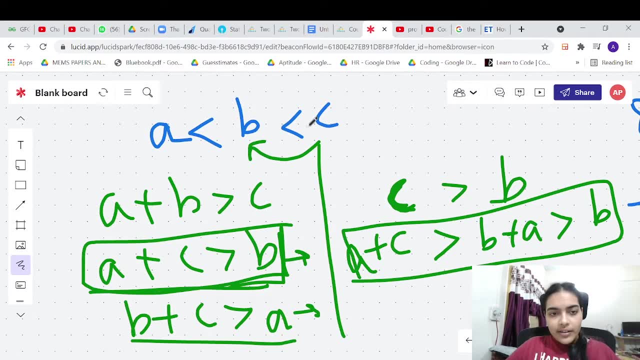 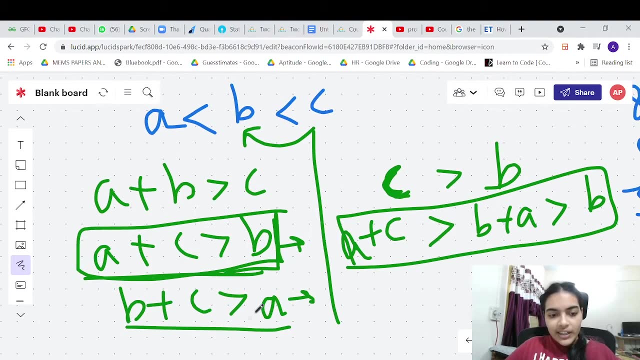 means c plus a is greater than b, right? So what does this mean? This means that this condition is going to be satisfied by default. If it is given that c is greater than a and b, right, Then this condition is going to be satisfied by default. okay, Similarly, the third condition is also: 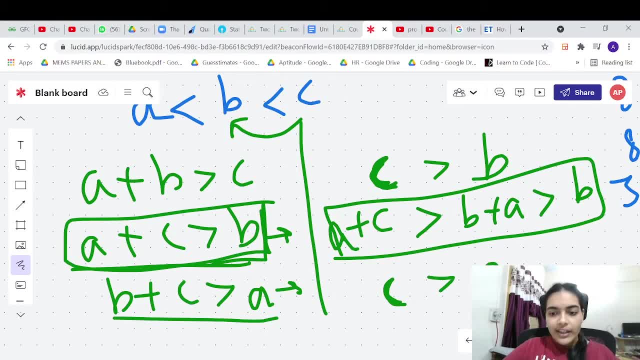 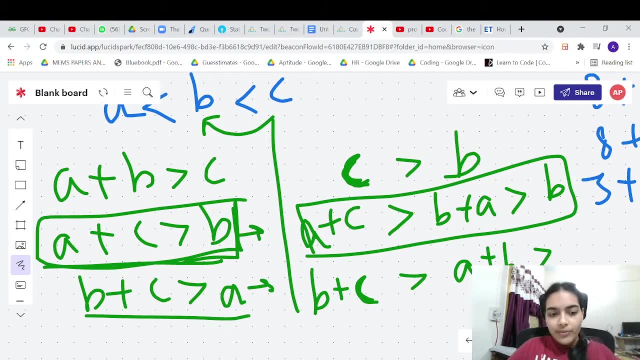 going to be satisfied by default. See, we know that c is greater than a right. So if I add b to both sides, c plus b will be greater than a plus b. That means that c plus b will be greater than a right. So this condition is going to be satisfied by default. These two conditions. 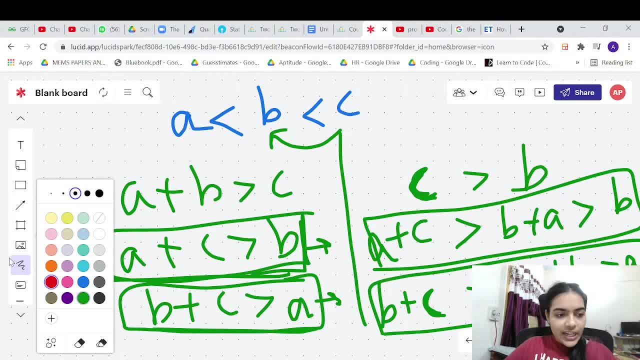 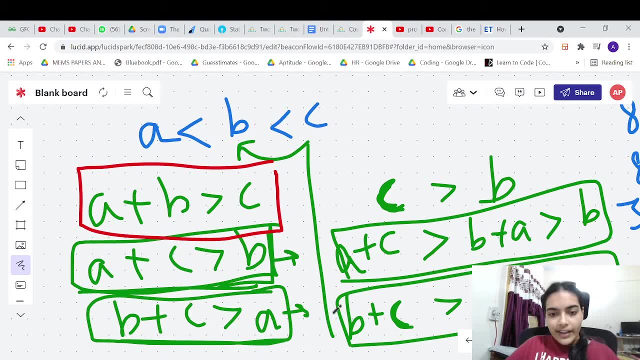 are satisfied by default. You only have a problem with this condition. You never know for sure whether this condition is true or not. Okay, Now, why is this? Why is this like this? Because, see, we know that third number is greater than, let's say, the first number, right? 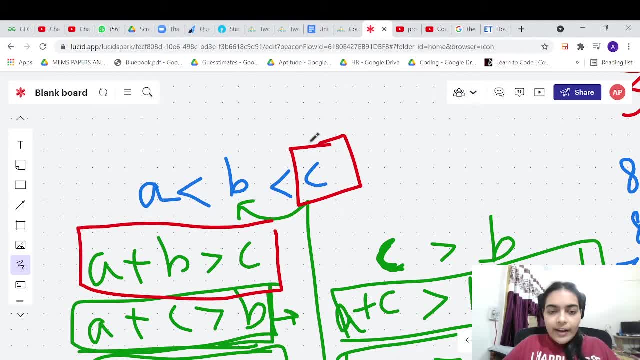 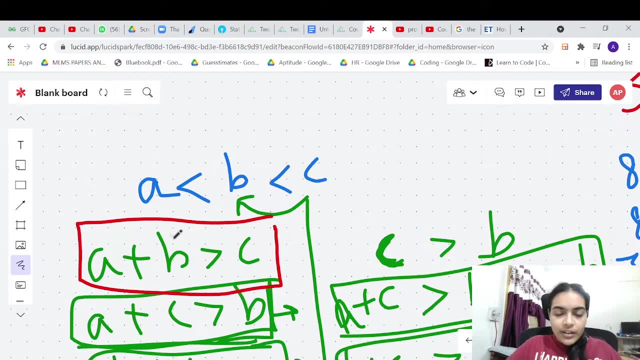 This is definitely known. So if you are adding third number to second number, that will also be greater than the first number, right? This is a simple logic. We know that third number, let's say third number- is definitely greater than first number, right? 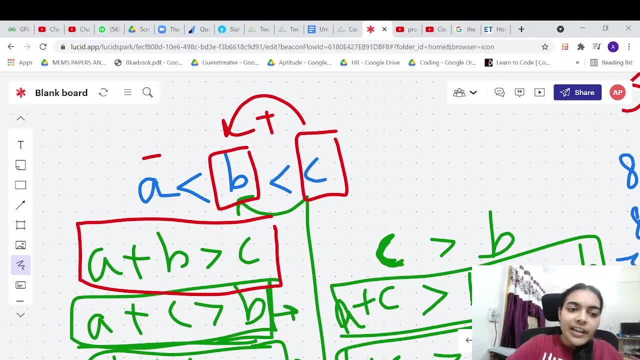 Now, if you add C and B right, that will definitely be greater than first number, because even the third number alone, single handedly, itself, it is greater than A. So C plus B, B is only helping it to increase its sum more. 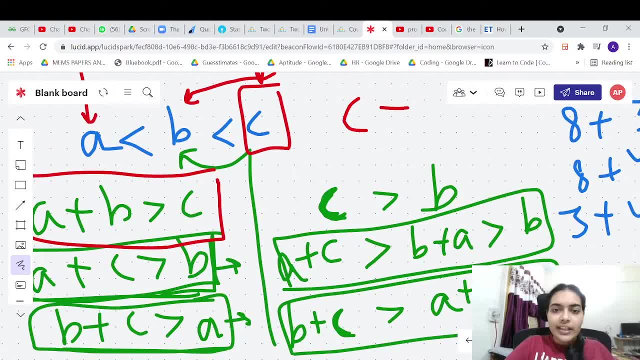 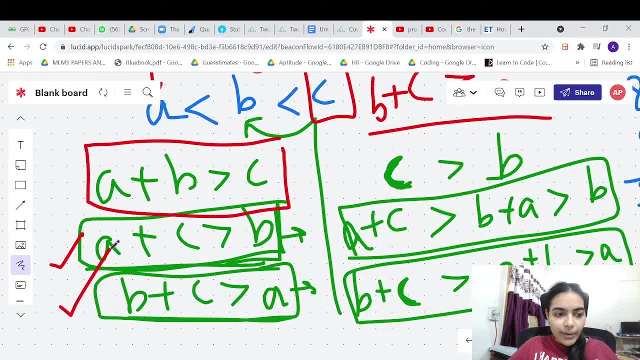 So C plus B will also be greater than A. We simply know that C is greater than A right, So C plus B will also be greater than A right. That's it. That is a simple logic. So these two conditions are going to be satisfied by default. 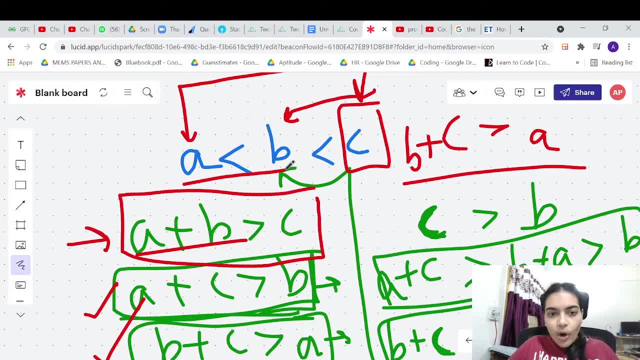 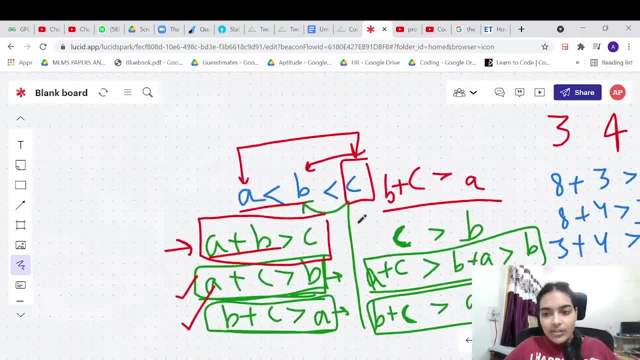 But this condition is doubtful, right? Which is this condition? Whether the smaller two numbers will add up to the third number or not. that is only the doubtful condition. okay, This is the simple logic in this question. Once we understand this logic, we will be able to solve the entire problem, okay. 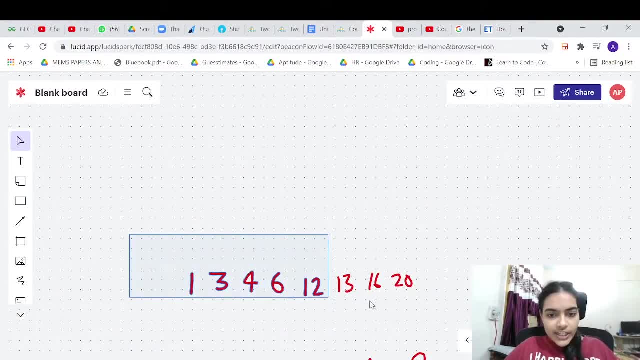 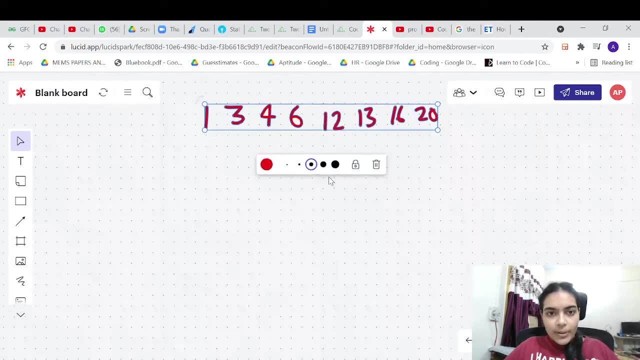 Now let's come back to our problem by taking that logic in mind. So let me copy this question and let's paste it here, okay? So now we have this question. Now let's try to see how many triangles we can form in this. 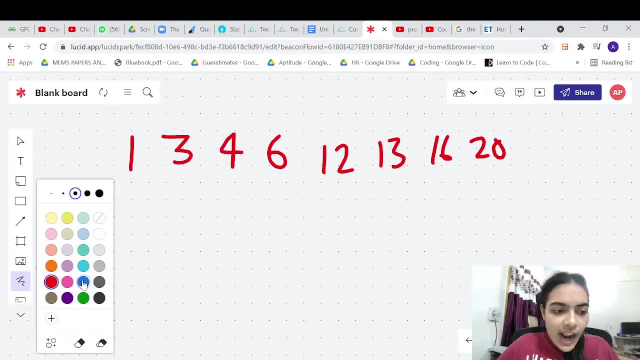 So now we know that if we choose the largest number right, We need not even check the conditions For the largest number. we need to only check the condition for the smallest number plus the middle number, Whether that will be greater than largest number. this is the only condition which is doubtful, right. 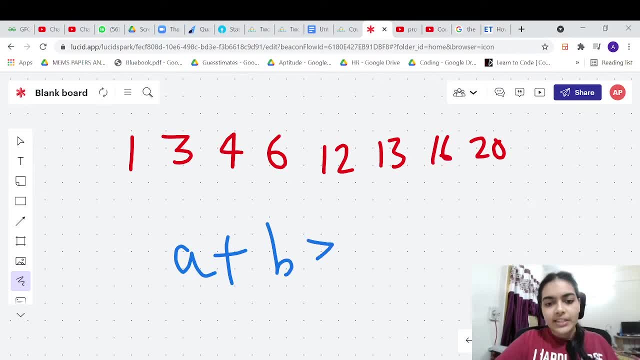 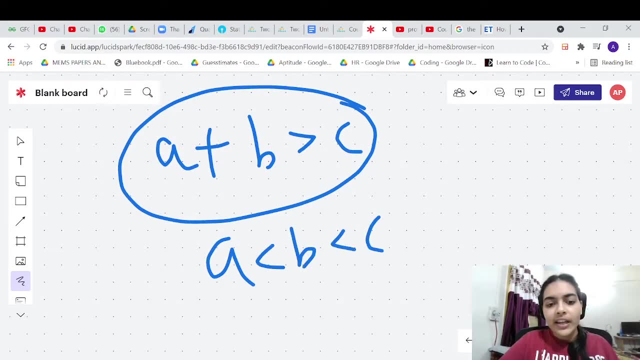 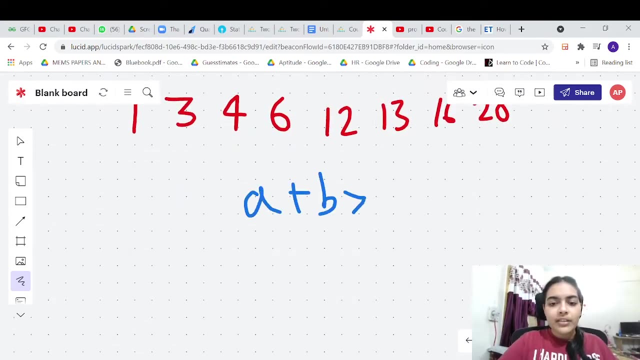 So the only thing that we need to check is A plus B is greater than C. We need not even check other conditions. If it is given that, if it is given that A is less than B is less than C, right, If it is given in this way, then we know that A plus B will be greater than C. 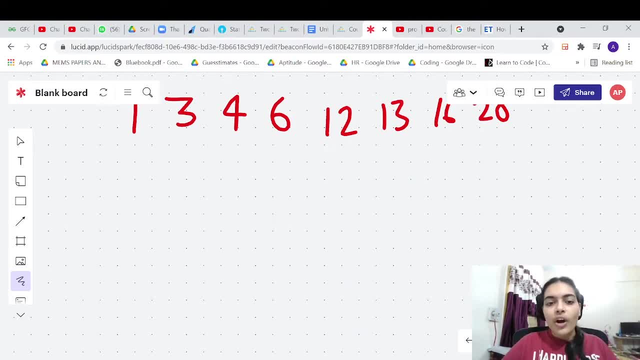 This condition is the only. This is the only condition. you need to check right. All other conditions- C plus A is greater than B. C plus B is greater than A- are going to be satisfied by default, Because it is given that C is greater than A and B. okay. 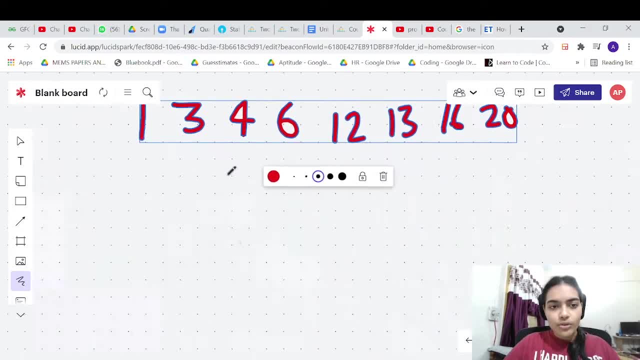 So that is the only thing we need to take care in this problem. Now let's try to solve this question, okay? So let's take the largest number now. Let's take the largest number and let's fix it right. 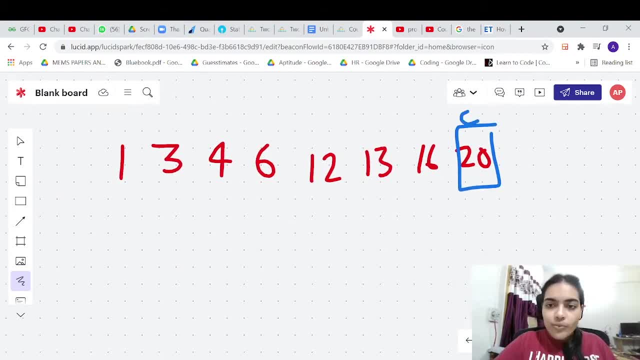 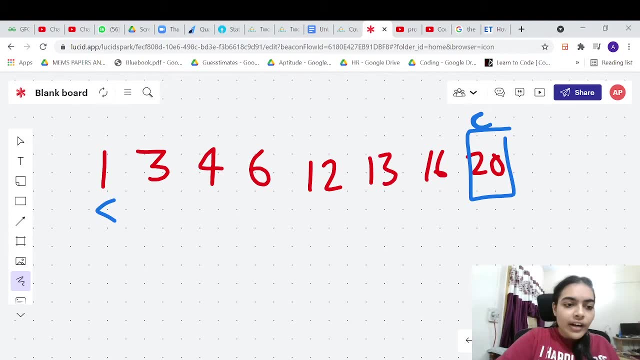 Because we know it's conditioned by default. So let's say: this is what we are fixing: our C. okay, We are going to fix our C and C is 20 for now. Now let's try to find out A and B among these values. okay. 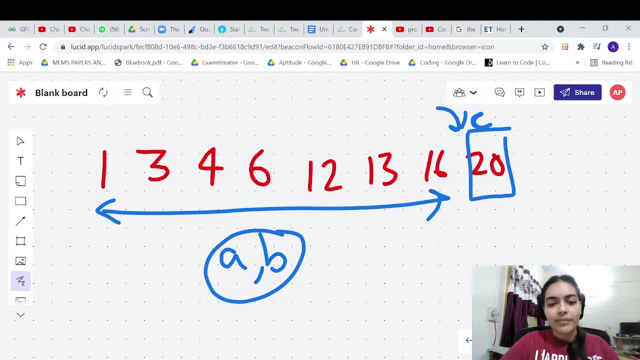 So we have fixed C. We are trying to find out A and B that will satisfy this condition. What is the condition that we need to check? The only condition we need to check is if A plus B is greater than C. okay, 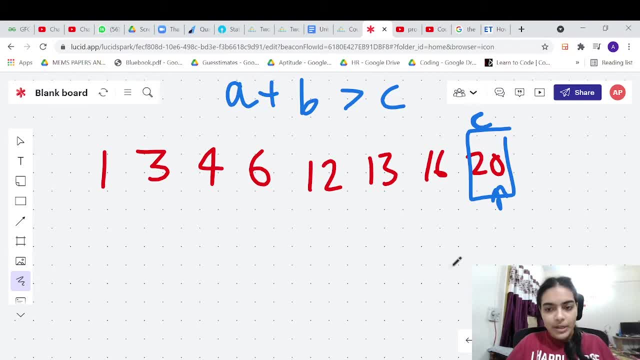 Other conditions will be satisfied by default, because C is the largest number. okay, Now let's start with. A is equal to 1 and B is equal to 16, okay, So A is equal to 1, B is equal to 16.. 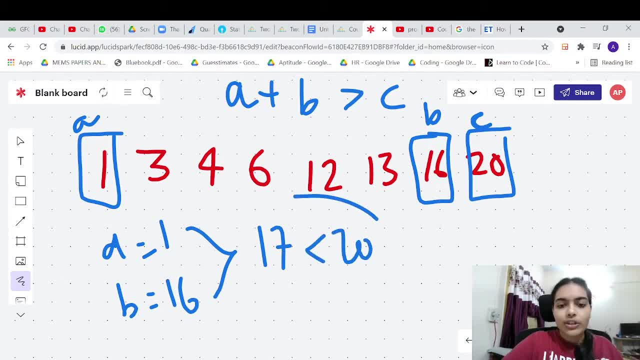 1 plus 16 is 17,, right, 17.. 17 is less than 20.. So the condition is getting violated, right? This condition is not getting satisfied. 17 is not greater than 20, okay. So what does that mean? 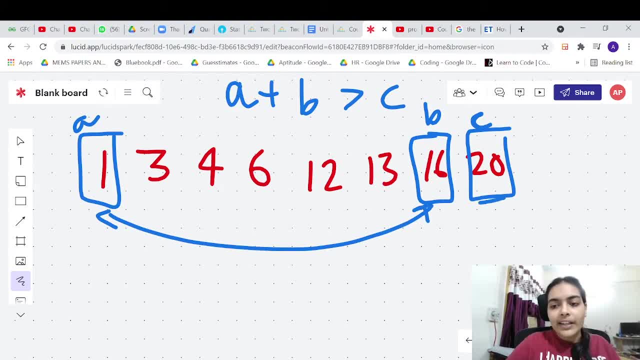 So these two numbers are not able to add up to be greater than 20, right, So we need to increase the sum of A plus B. right, We need to somehow increase our sum. okay, So that's a very bad increase arrow, but let me try to draw it again. 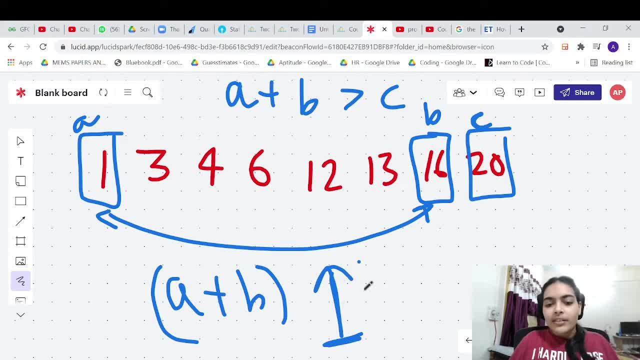 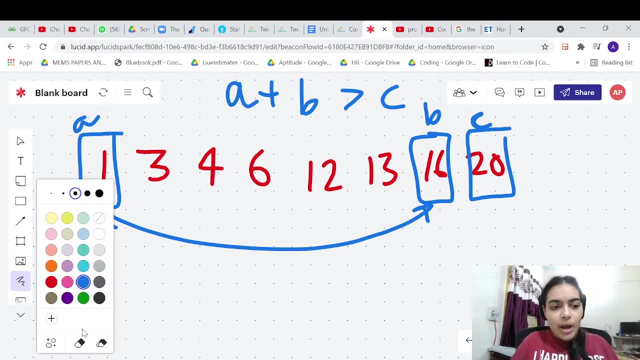 So we need to increase our sum to try to make it bigger so that it can satisfy. So we need to simplify this condition, because right now our sum is less right, So we need to increase the sum. How will you increase the sum right? 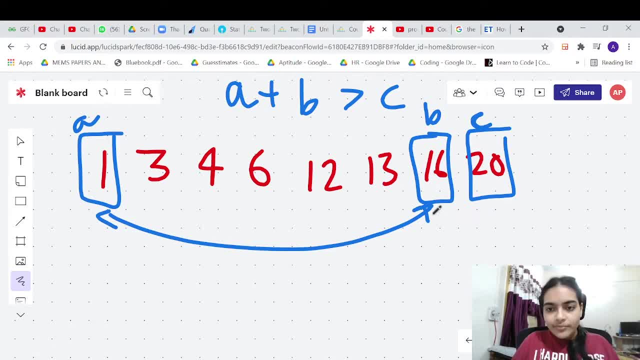 You cannot stretch on the right side, because right side we cannot take any value greater than 16, right We have to take values only from 1 to 16.. So how can we increase the sum? You can try to increase A. 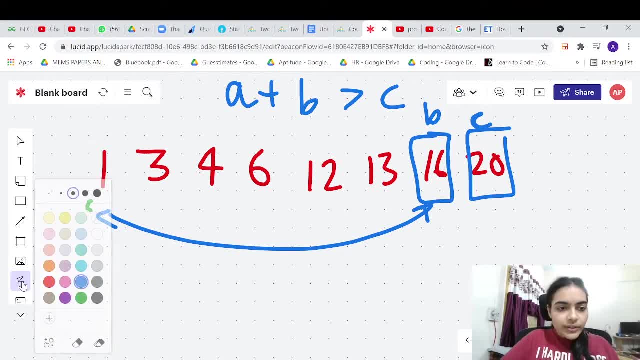 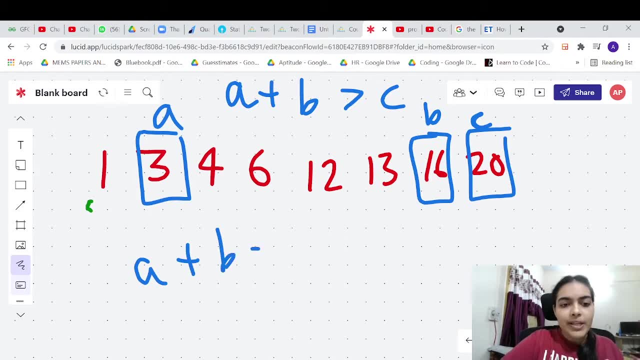 It is sorted in ascending order, right? So if you move A, you only have the option of moving A, right? You can increase the sum by moving A, So let's move A, okay? So in this case now, what is our A plus B? 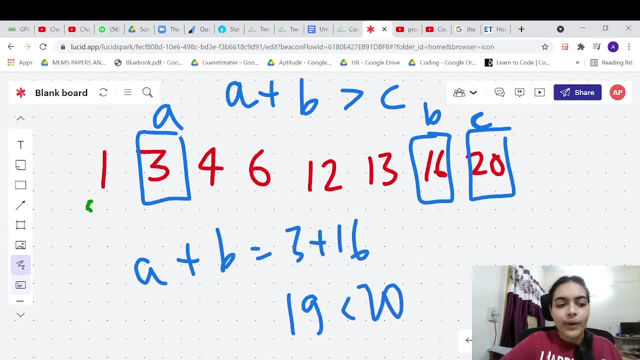 3 plus 16.. 19. 19 is still short of 20, right 19 is still shorter than 20.. It is still smaller than 20.. So in this case again, we are not able to satisfy the condition. 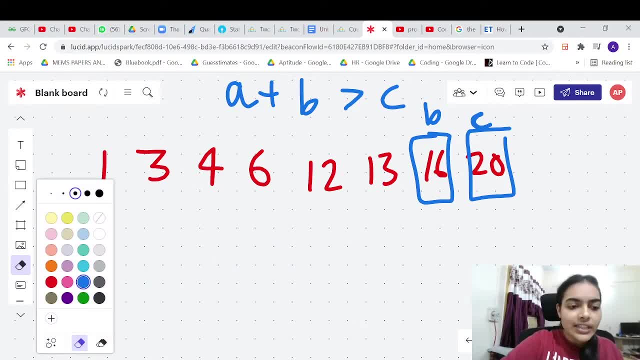 The condition is getting violated. So now again, we have to try to increase our A plus B, right? So we have to try to increase our A plus B. How can you do that? You can try to do that by increasing A. 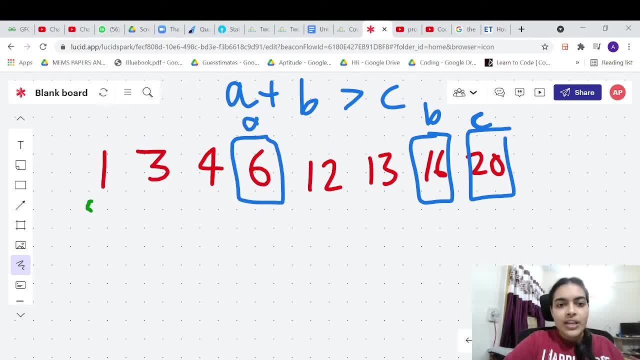 You cannot move B because B is already in the end, right In this case. So let's try to shoot up our A. Sorry, A will come here: 4 plus 16.. 4 plus 16.. 16 is still not greater than 20,, right? 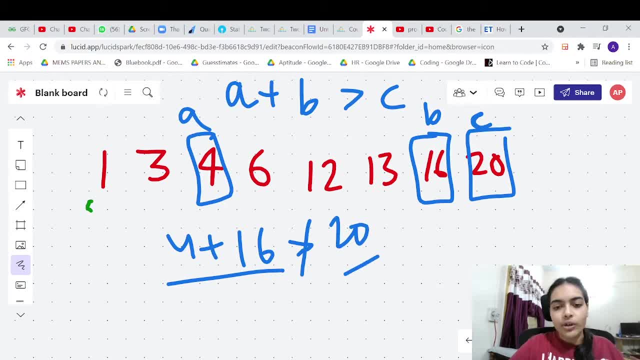 4 plus 16 is 20.. 20 is not greater than 20, right. So again the condition is getting violated. So we need to still increase our A. So let's try to move our A: 6 plus 16.. 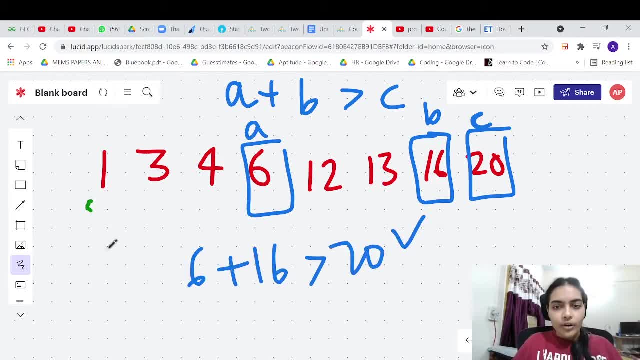 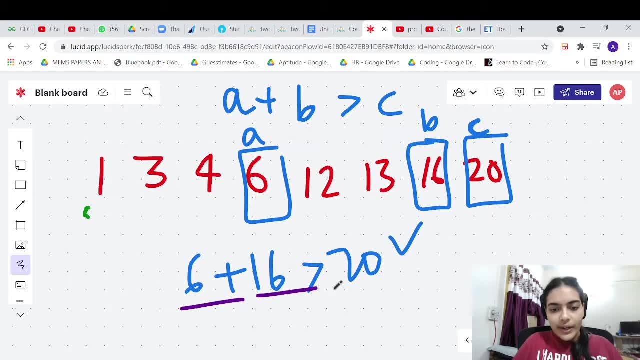 22 is greater than 20, right Now, the condition is getting satisfied. Okay, So now, for the first time, we are able to form a triangle using these three values. What are the three values? 6,, 16 and 20, right. 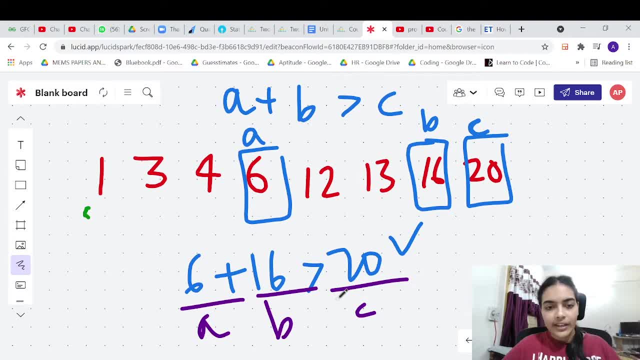 We have taken A, B and C in this order: 6, 16 and 20.. We are able to satisfy and form a triangle, So let me Keep a count variable. Okay, So count is equal to 1.. 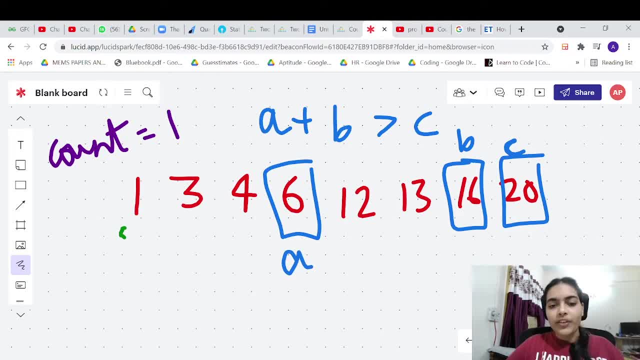 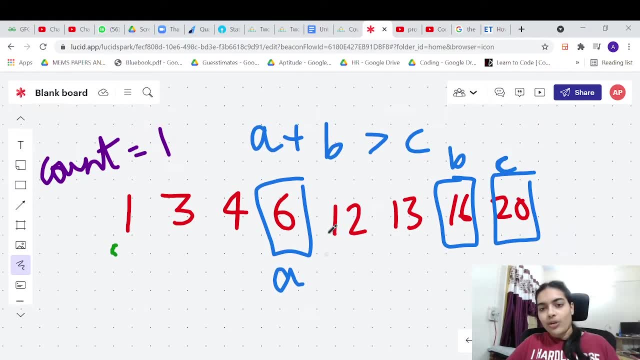 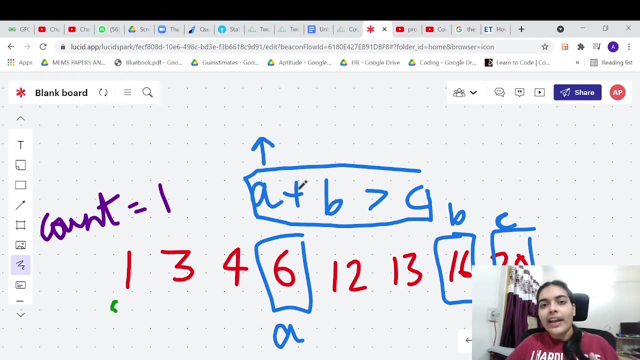 Okay, Now again one very important concept we have come to here. Now see: If I move my A, I will get further answers. also, See: A plus B is greater than C, right, If I move my A, if I increase my A now, I will definitely get. 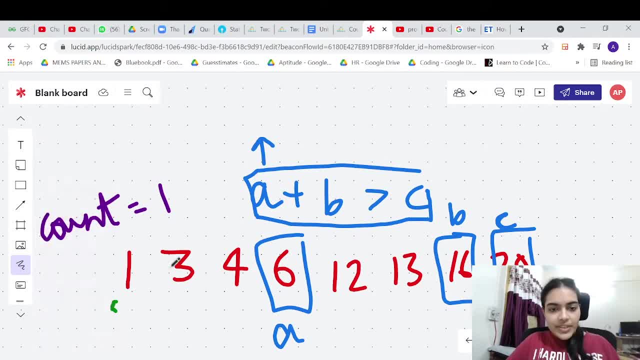 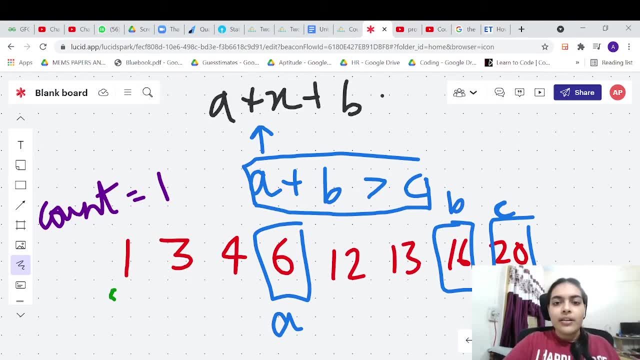 I will definitely satisfy this condition. See, The logic is simple: A plus B is greater than C, right? Let's say I take a value which is little greater than A. Let's say I take A plus X, Okay, Well, X is a value, just little greater than A, right? 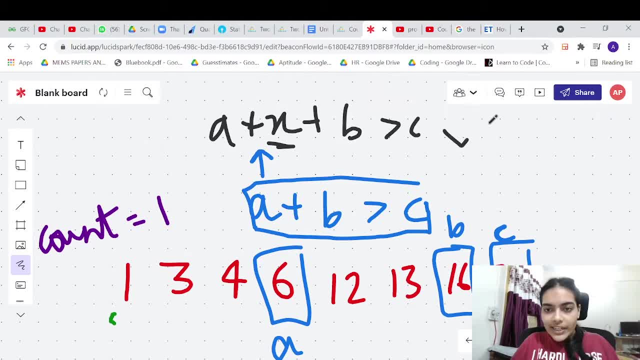 We are moving this side, So this will definitely get satisfied. because this is satisfied. A plus B is greater than C, So any value, if you take greater than A, that will also add up and increase your sum and satisfy this condition. 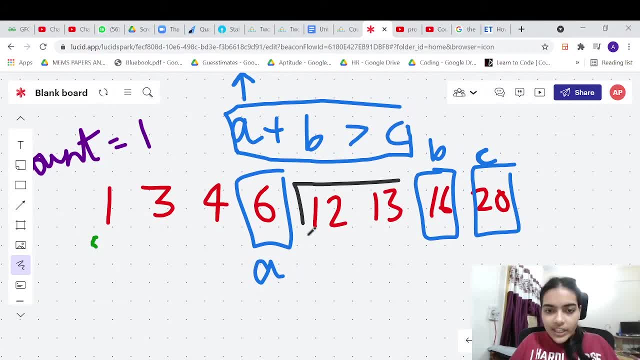 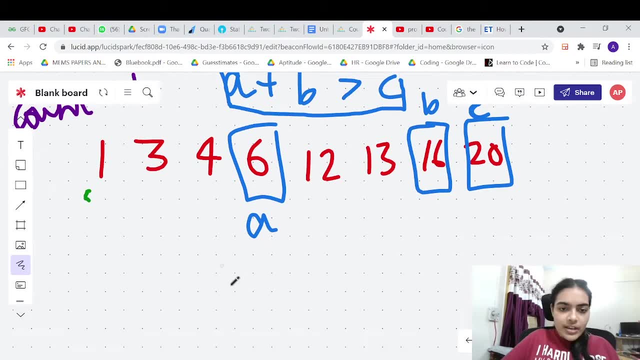 So what does that mean? Do I even need to check for these values? I need not even check for these values, right? Because by default, these two conditions are going to get satisfied. See: 6 plus 16 is greater than 20, right? 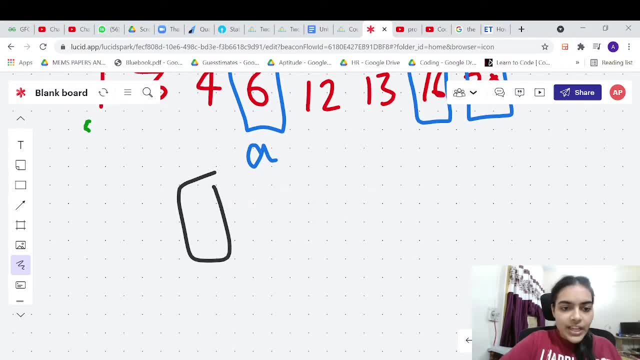 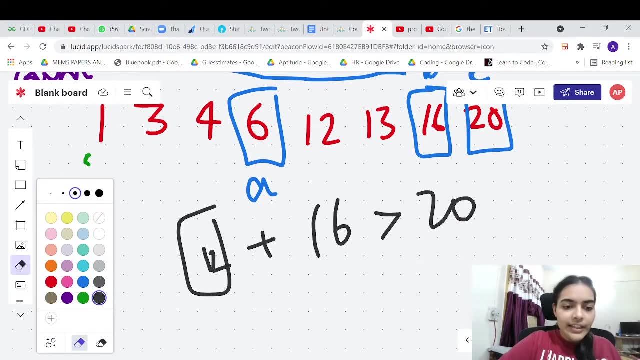 So if I increase my A right, If I change my 6, instead of 6, I take 12.. 12 plus 16 is also going to be greater than 20, right, If instead of 12, I take some other value which is greater than 12, okay? 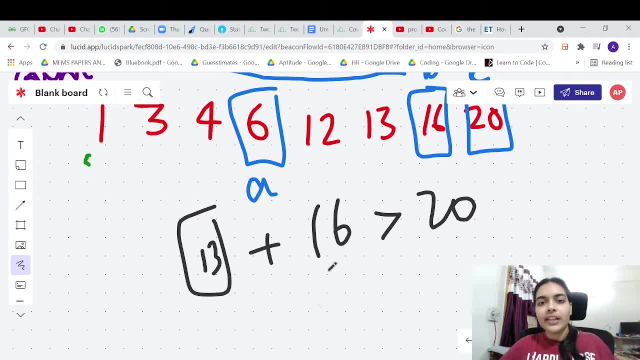 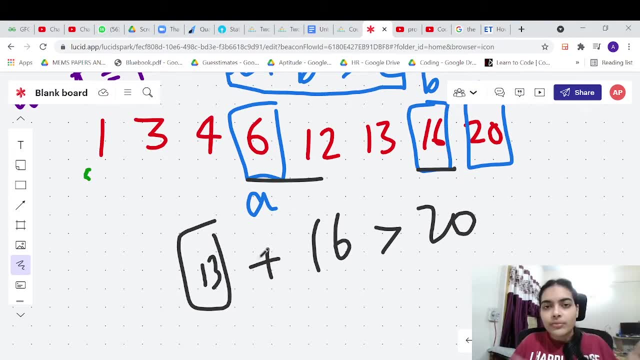 I take 13.. 13 plus 16 is also greater than 20, because 6 plus 16 is itself greater than 20.. Smaller number itself is giving you a large enough sum. So any number greater than 8.. So any number greater than 8 will anyway give you the sum. 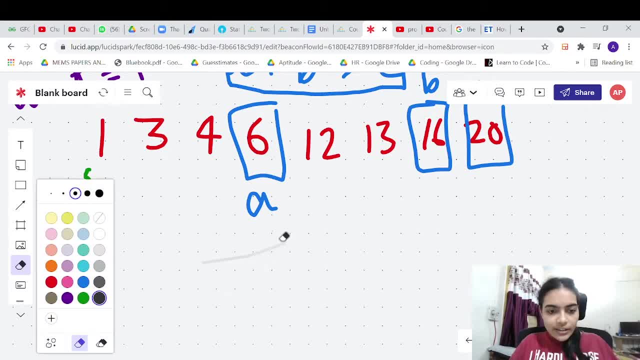 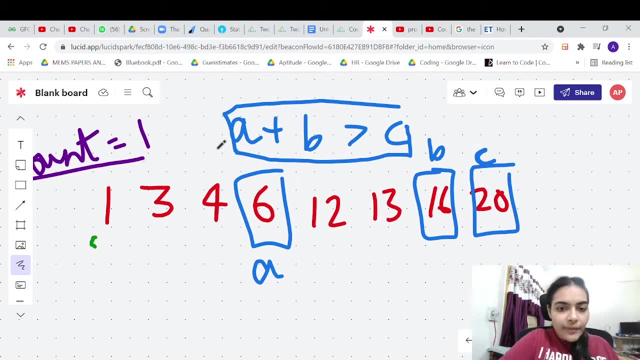 So what does that mean? Now, once we have reached the limiting condition where, first time we are satisfying, A plus B is greater than C, you can increase your count, right. You need not even check for other A values. You need not check for these values of A. 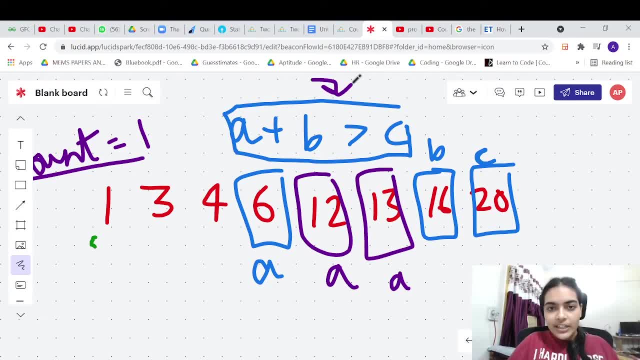 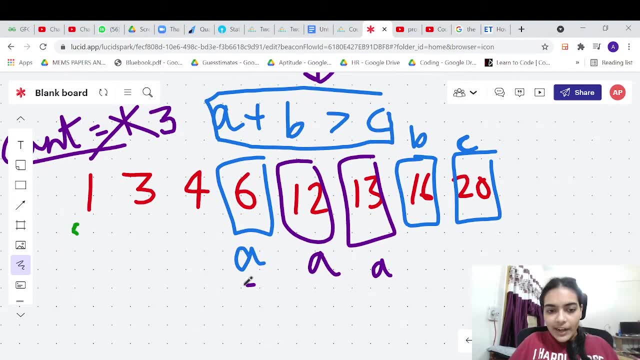 Okay, They will anyway be greater and satisfy this condition, So count can be directly made to 3.. Okay, What is 3?? 3 is the difference between B and A. Okay, 3 is the difference between B and A. 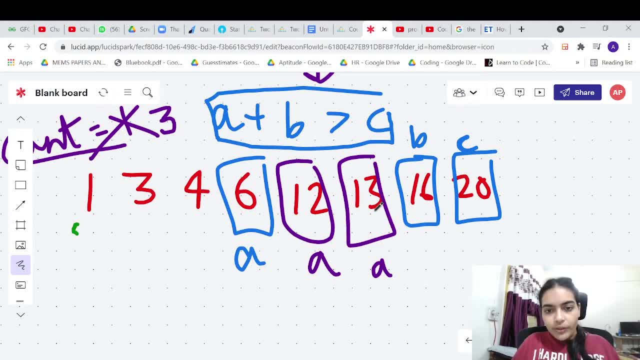 So B is at index Number 0,, 1,, 2,, 3,, 4,, 5, 6,. right B is at index number 6.. A is at index number 3.. There are 3 values between A and B. 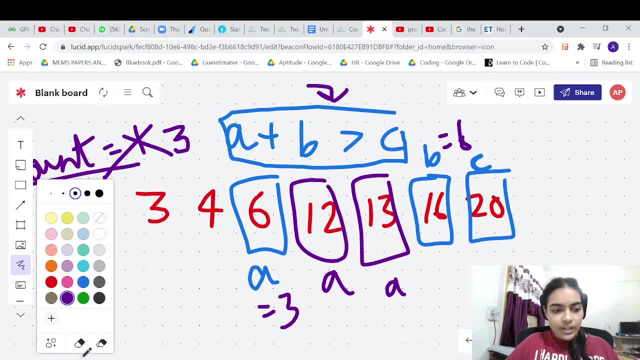 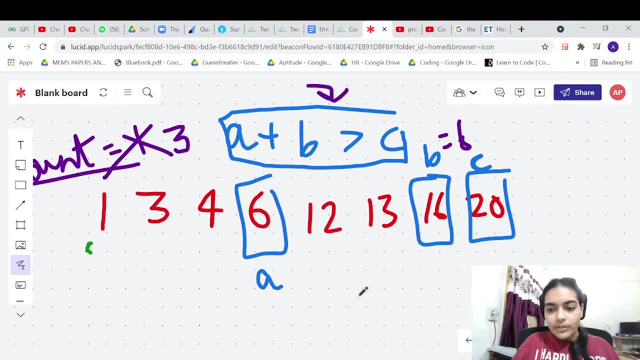 So you can take all these 3 values will satisfy this condition. Okay, So now I need not move my A. What do I need to move then? I need to move B. right Now I need to move B and try to see if it is satisfying the condition. 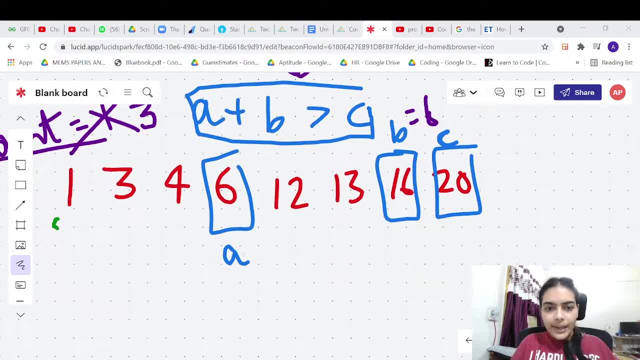 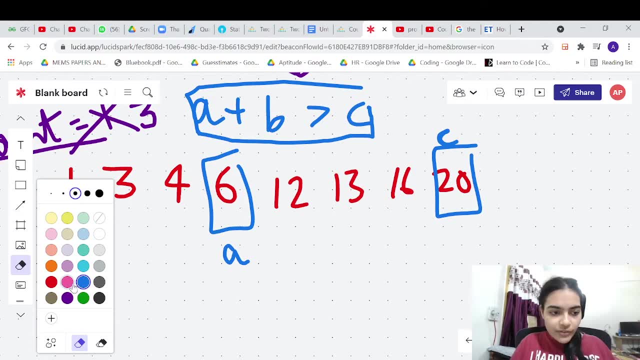 So I have moved A. Okay, I need not move A, So I will move B. Okay, Now I will move B For the first time. I am shifting my B, I am decreasing my B And B comes here. 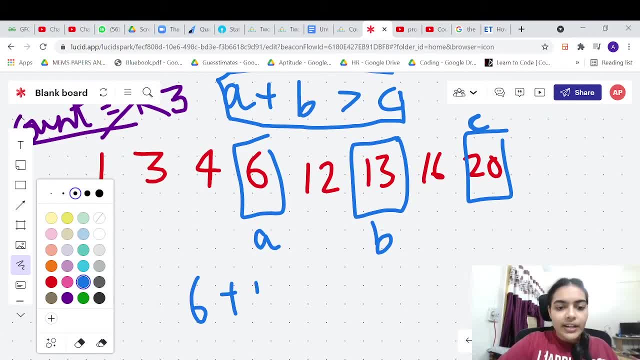 Okay, So in this case you have 6 plus 13.. Now you are trying to check if 6 plus 13 is greater than 20.. 6 plus 13 is 19.. 19 is less than 20, right? 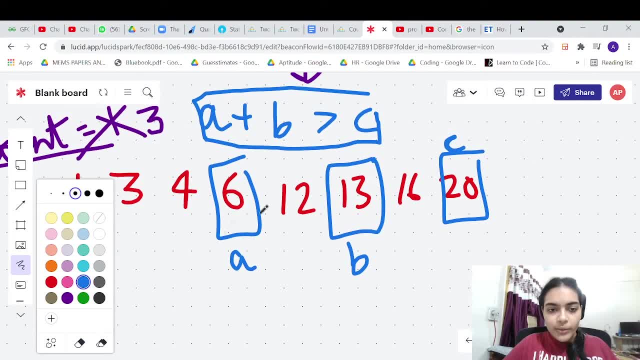 So in this case, you are not satisfying the condition. So what do you need to do? You need to again move your A now. Okay, Because we are falling short. So you need to move A. So you come here. 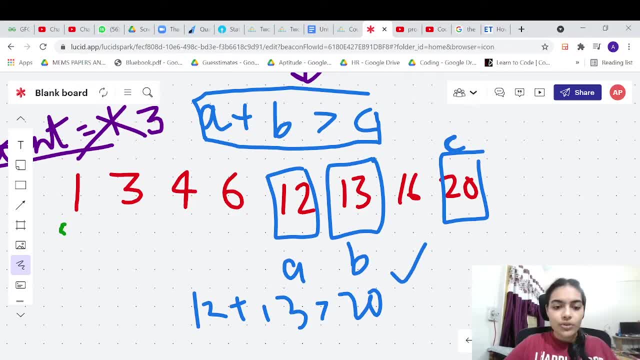 12 plus 13.. 12 plus 13 is greater than 20.. This condition is true, right? 12 plus 13 is 25.. 25 is greater than 20.. So I can change my count. So my answer will be 4.. 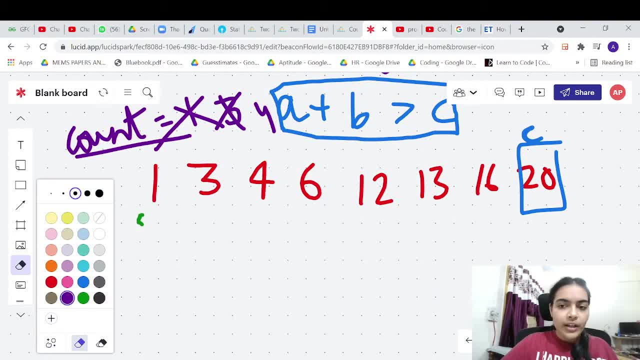 As of now, I have found one more triangle. Okay, Now let's go forward. So we have finished all the iterations. Okay, We have found all the possible values of A and B that were possible by keeping C fixed. Now let's try to change C. 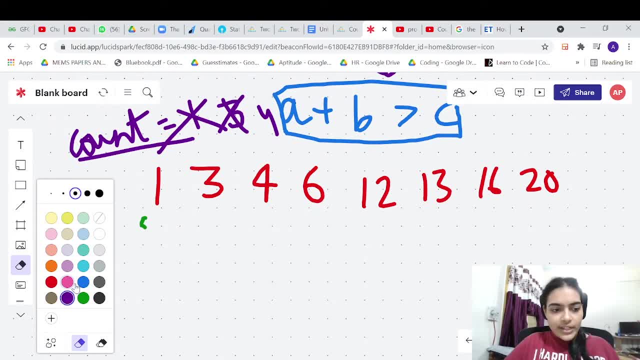 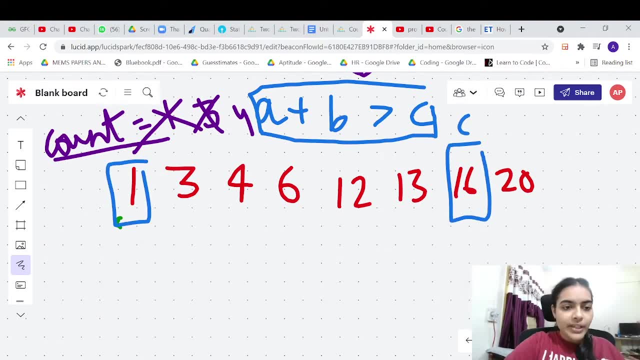 And let's try to see if we can find some other values. Okay, So now let's try to change our C, So C is 16.. Okay, Again, let's try to start. Let's start from here. A is 1.. 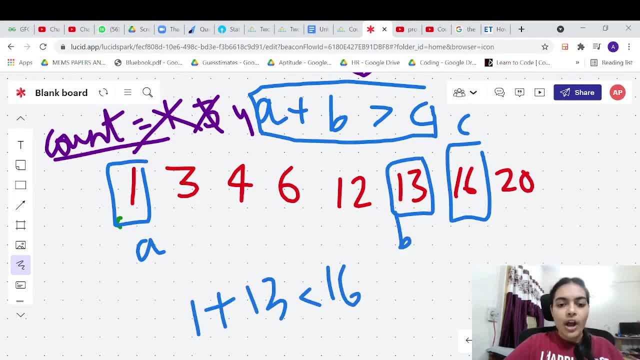 B is 13.. Okay, 1 plus 13 is less than 16.. So now I am falling short, I need to increase my A. Okay, So whenever I am falling short, I will increase my A. So let me try to move up my A. 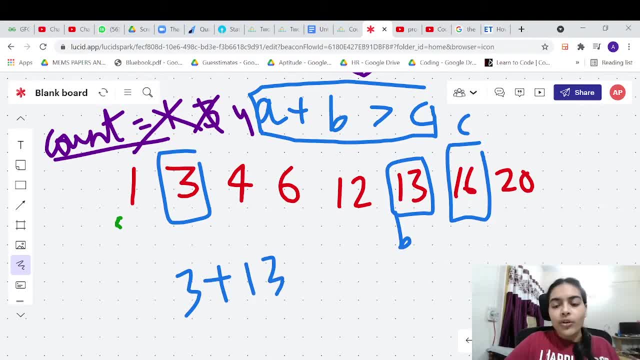 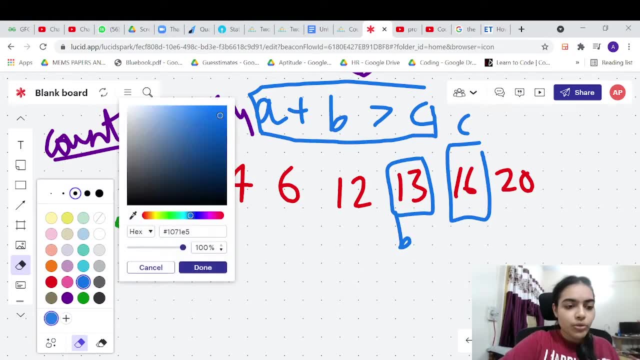 So in this case, 3 plus 13 is again not greater than 16.. Right, When I compare them, both are equal, But it's not greater than 16. So I need to still move my A. So I will move my A to the next value. 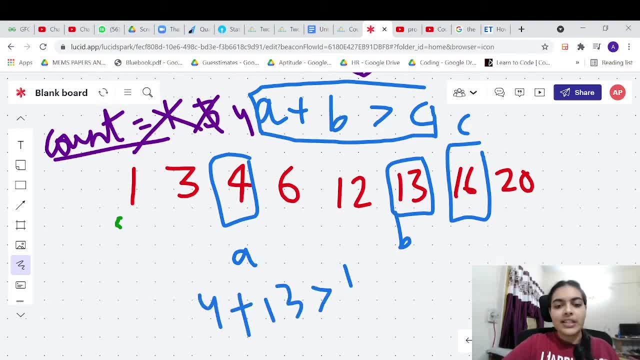 Now, A is 4.. B is 13.. 4 plus 13 is greater than 16.. Okay, 4 plus 13 is greater than 16.. Right, So this condition is satisfied. So all these conditions will be satisfied. 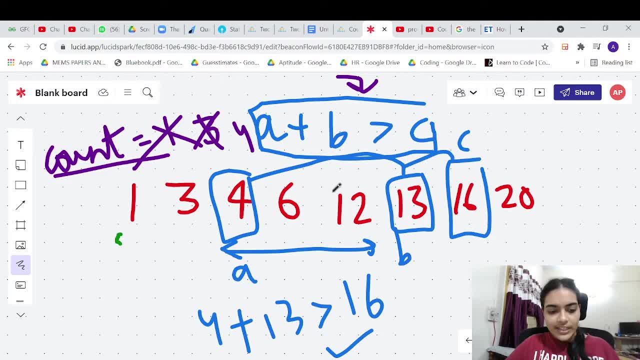 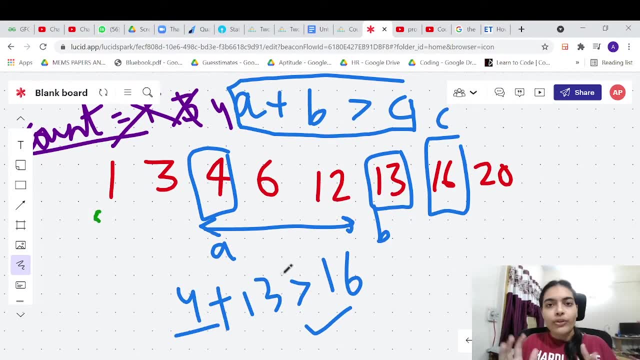 I will get 3 triangles directly. 4 plus 13 is greater than 16.. 6 plus 13 is greater than 16.. 12 plus 13 is greater than 16.. So once I find an A value, I need to check for other A values with the same B and C values. 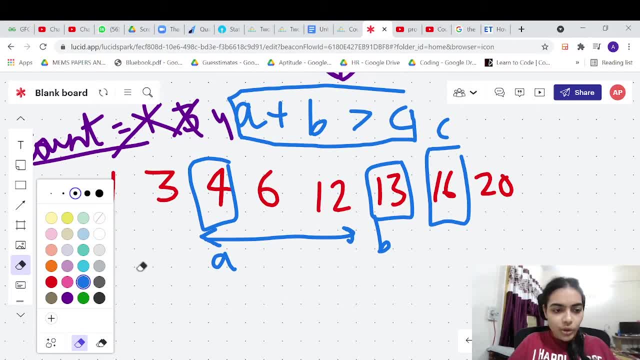 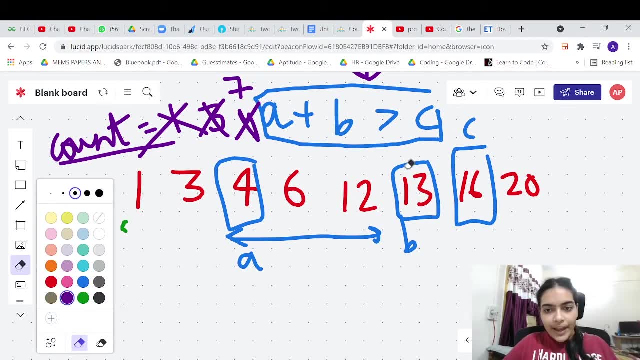 Right. All other remaining A values will get satisfied. So I have found 3 more triangles. So now my count will increase From 4, it will become to 7.. 4 plus 3 is 7.. So now I will shift my B value. 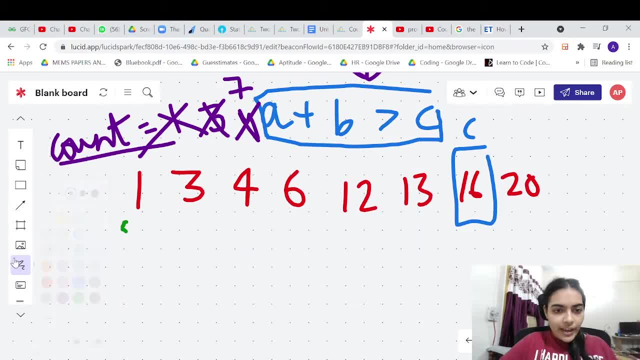 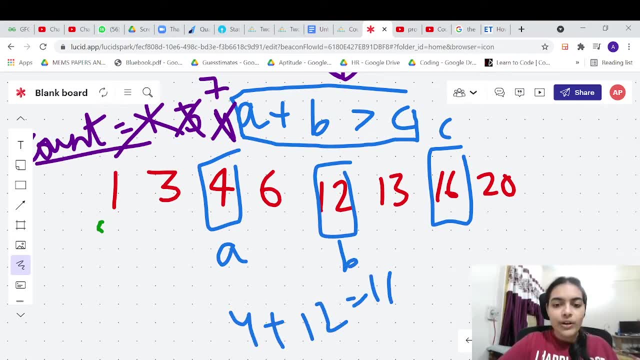 Okay, From 4, I will try to shift my B value. So I will keep my A fixed and I will try to shift B. Okay, So in this case, 4 plus 12 is 16.. 16 is equal to 16,, not greater than 16.. 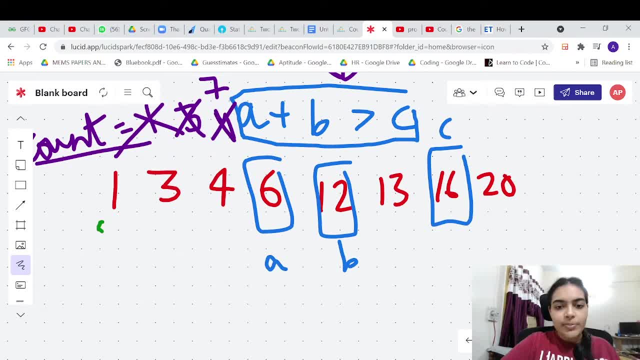 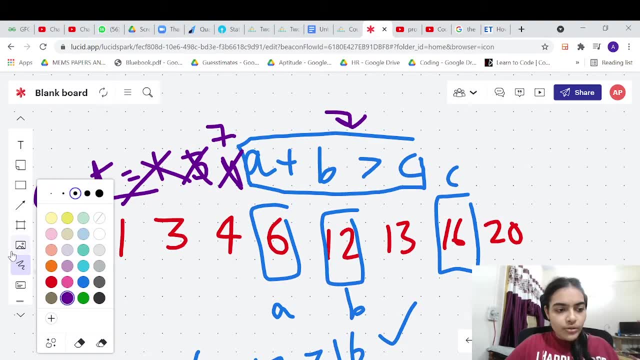 So I need to increase my A value again because I am falling short. So 6 plus 12 is greater than 16.. Right, 18 is greater than 16.. So the condition is getting satisfied. So I need to change my count. 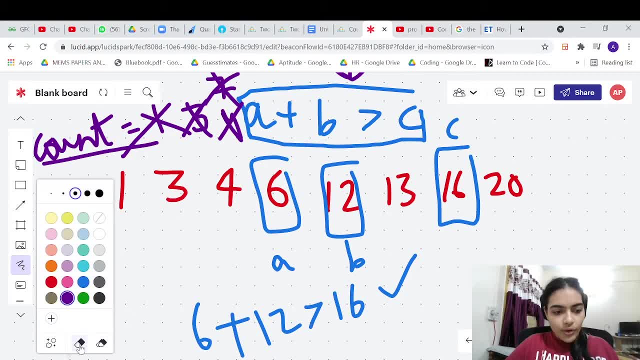 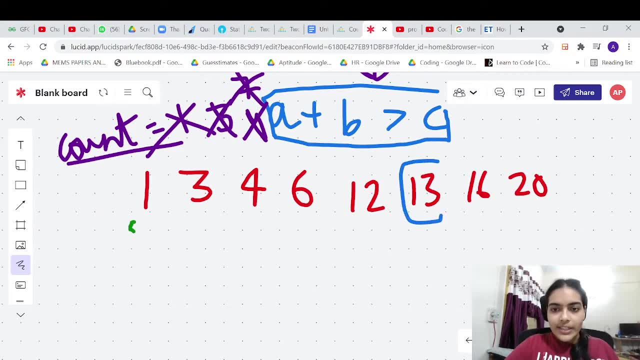 So count will become equal to 8.. Okay, Now let's go forward to the next value. Now, with this possible C, I have exhausted all possible solutions, So let's move my C up here, Okay, So in this case, C is 13.. 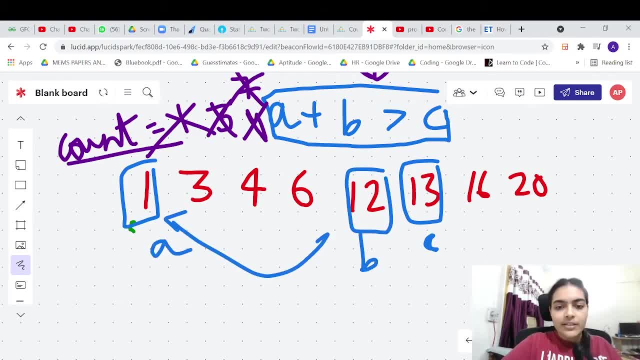 I will again bring my A and B values. 1 plus 12 is 13.. 13 is equal to 13,, not greater than 13.. So I need to shift my A value. So 3 plus 12 is 15.. 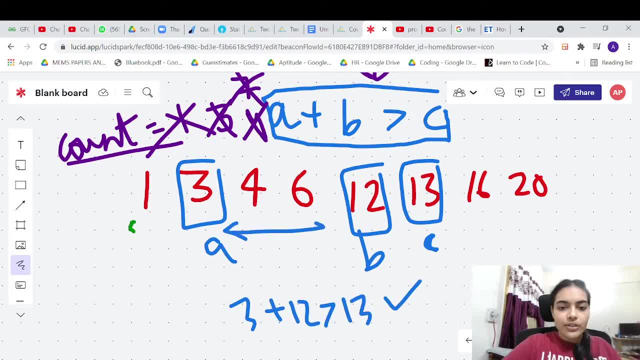 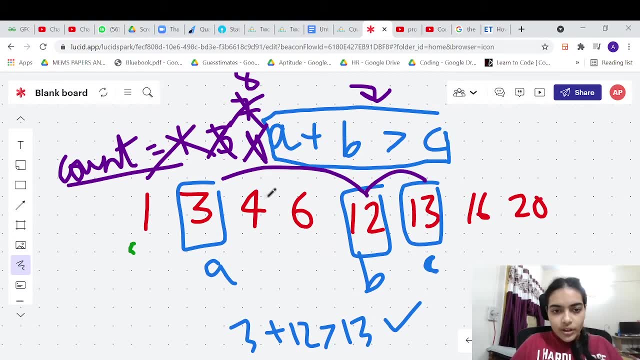 15 is greater than 13.. So I have satisfied the condition. So all these three cases will satisfy the condition. Right, 3 plus 12 is greater than 13.. Okay, So even 4 plus 12 will get satisfied. 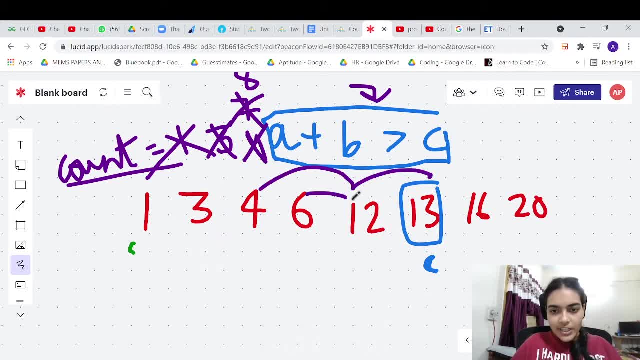 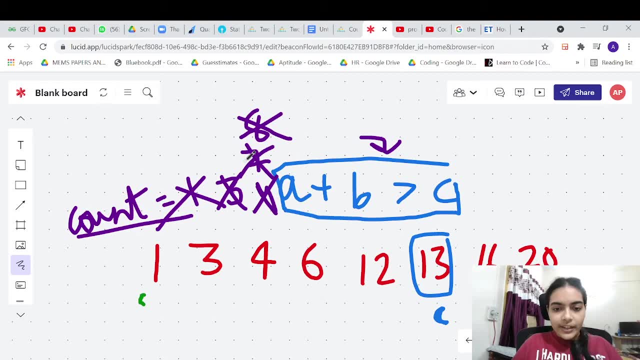 Okay, 6 plus 12 will be greater than 13.. 16 is greater than 13.. And 6 plus 12.. 18 is also greater than 13.. Right, All these values will get satisfied. So I have again found 3 triangles. 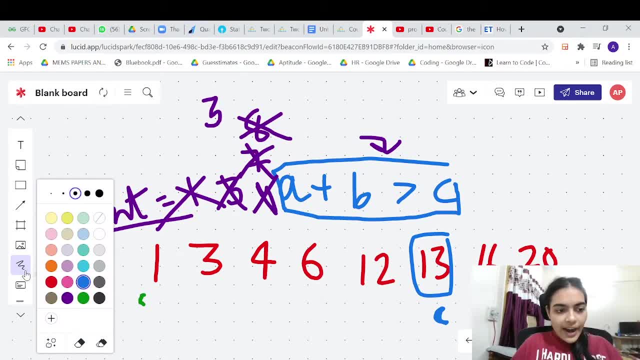 Right. So I have again found 3 triangles, So I will add 3.. So 8 plus 3. Right, 8 plus 3 will become equal to 11. So my count will be 11.. 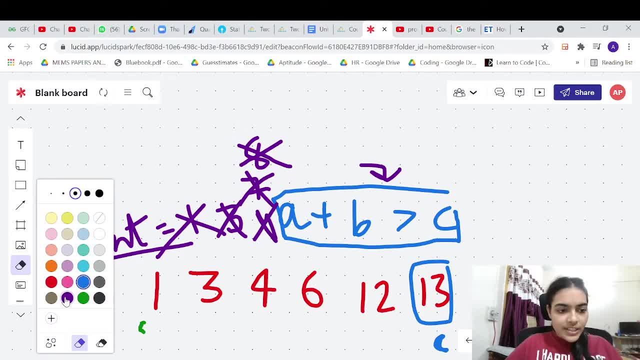 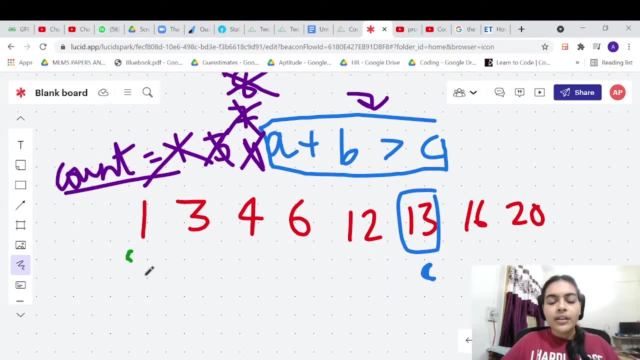 Let me write it properly. Count will be 11.. Count was earlier 8. It will become 11.. Okay, Now I again need to shift my C. Okay, So what was my last A and B that I saw? 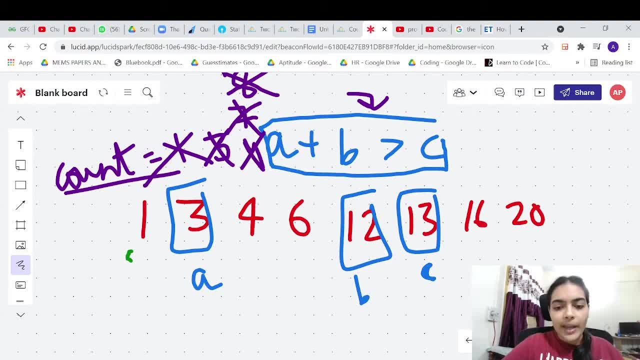 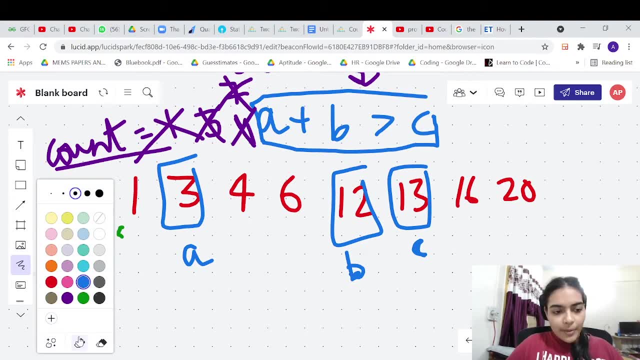 So my B was 12 and my A was 3.. Right, So I found A plus B greater than C. So I took all these three values Right, And now I will try to shift my B. So in this case, I will try to shift my B. 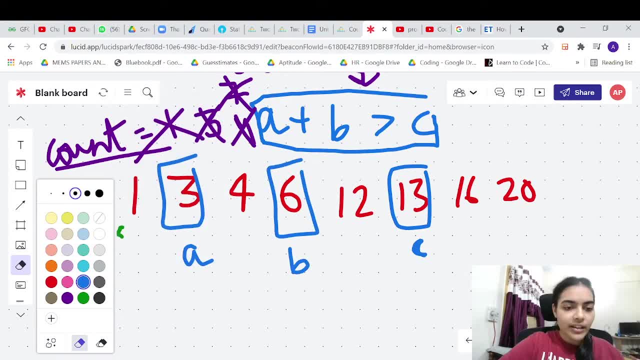 So in this case, 3 plus 6 is 9.. 9 is less than 13.. So I will again try to shift my A: 4 plus 6.. 6 is also less than 10.. 10 is also less than 13.. 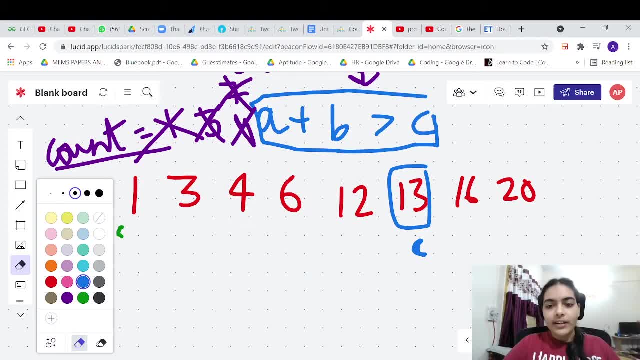 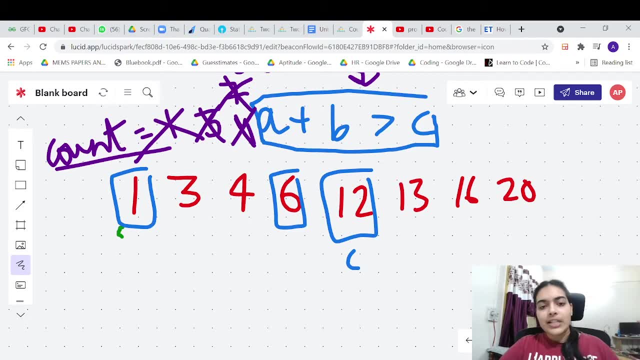 So I have exhausted all possible values Right. So now I will shift my C back again, So in this case C is 12.. I will start from these values: 1 plus 6.. 6 is 7 is less than 12.. 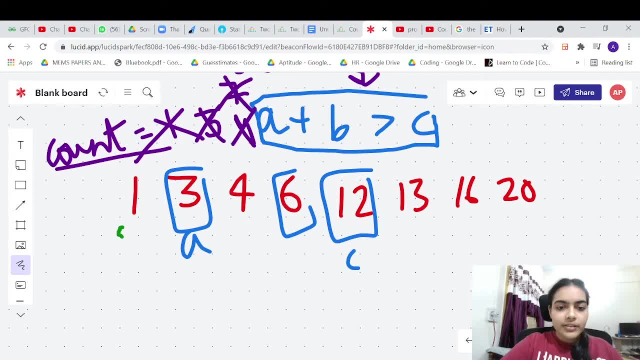 Right. So I will try to move A 3 plus 6. 9 is also less than 12.. So I will try to move my A 4 plus 6. 10. 10 is also less than 12.. 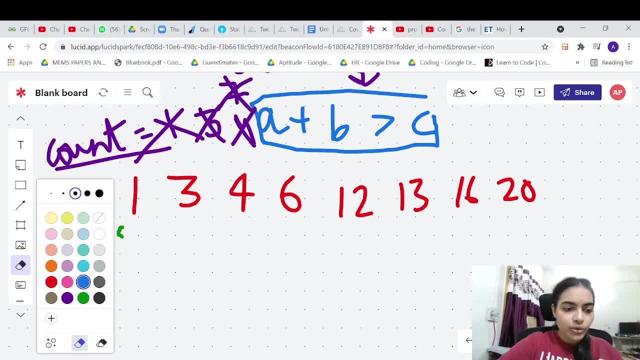 Right, So I will. I have not found any possible value, So now I will again move my C. So C is 6.. 1 plus 4 is 5.. 5 is not greater than 6.. Okay. 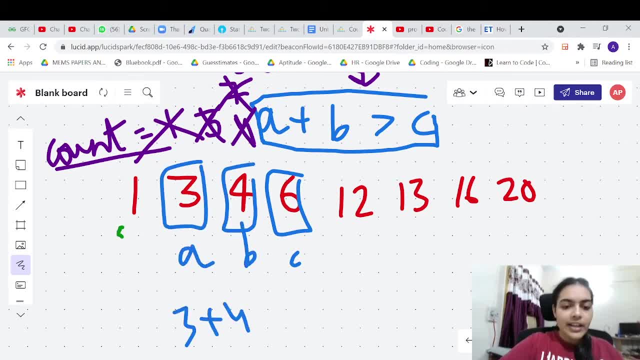 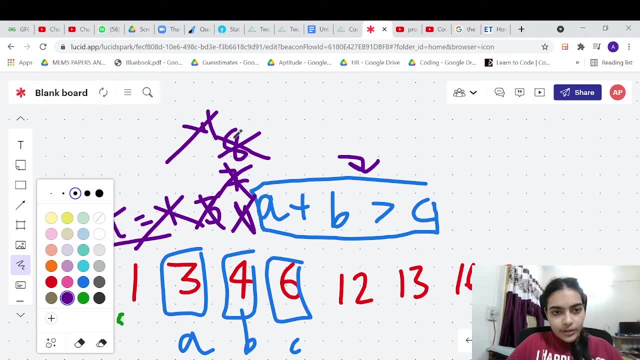 Now, 3 plus 4 is 7.. 7 is greater than 6.. So I have again found one more triangle, So let me shift my count. Count will become equal to 12 in this particular case. Okay. 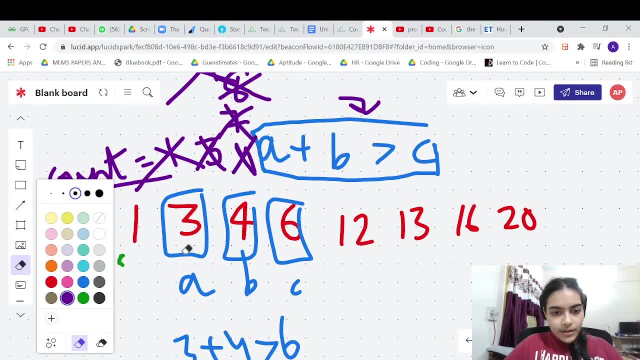 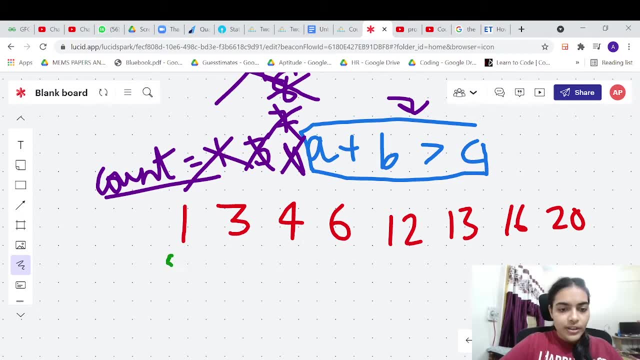 Count is become equal to 12.. So now let me move my C value. So this is the last C value that I need to take, Because I need to have at least 3 values, Right? So in this case, I will check. 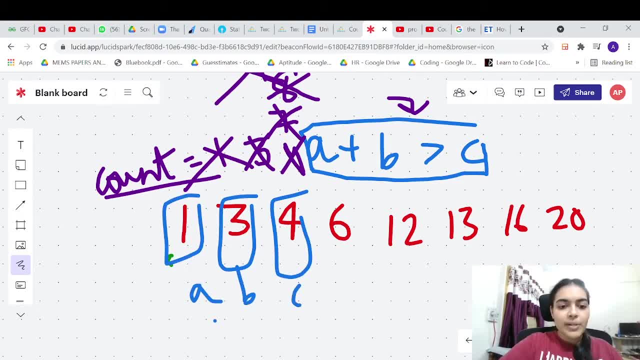 1 plus 3.. These are my A, B, C values. 1 plus 3 is 4.. 4 is not greater than 4.. Right, So I will not be able to form a triangle, So I have finished all my values. 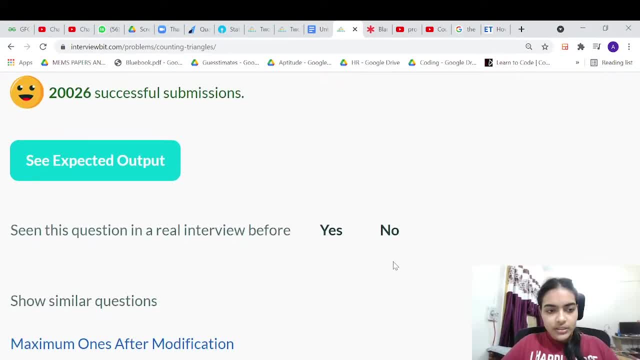 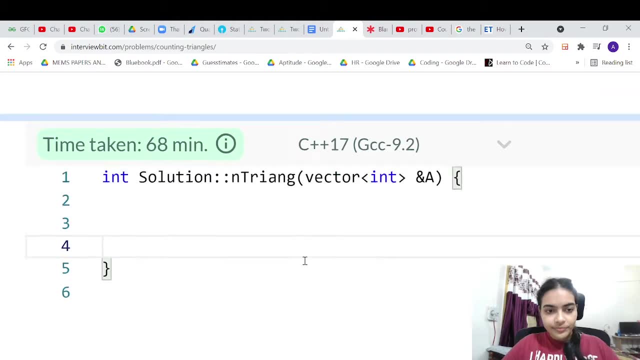 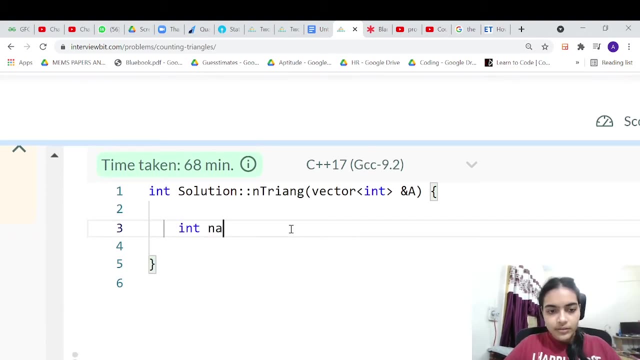 And my count is 12.. 12 is the answer. Okay, Now let's move forward to coding it. Okay, Let us start coding it. So let me declare int answer Okay And let me initially make it 0.. 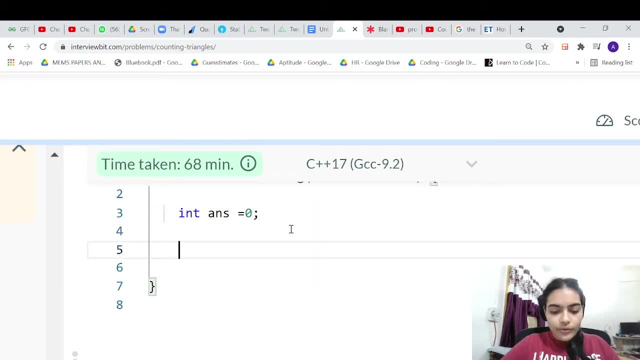 Okay, Now let's try to form the triangle. So we have to take 3 values Right- A, B, C- for triangle that satisfy the given condition. A plus B greater than C, Where you know, A, B, C are sorted. 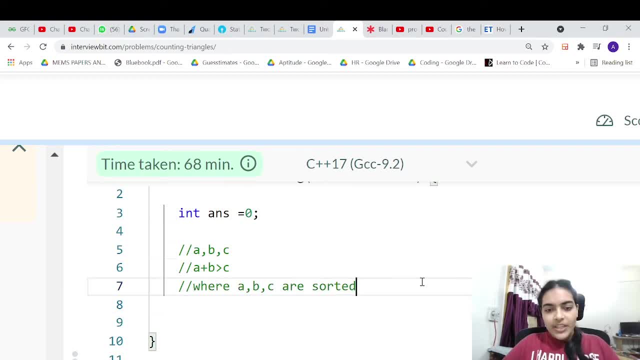 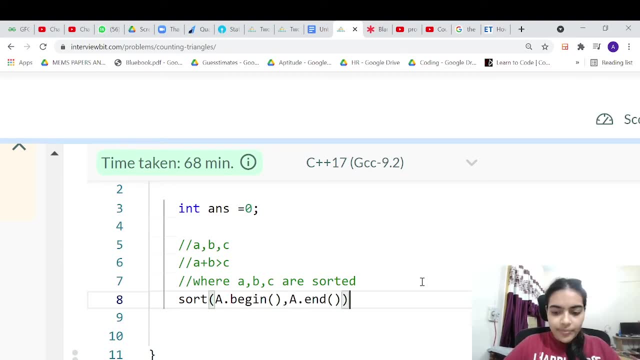 Okay. So this is the simple logic of this question. So let's first sort A. So sort A dot, begin A dot, end. Okay, So we have sorted it. Now let's try to fix C. Okay. 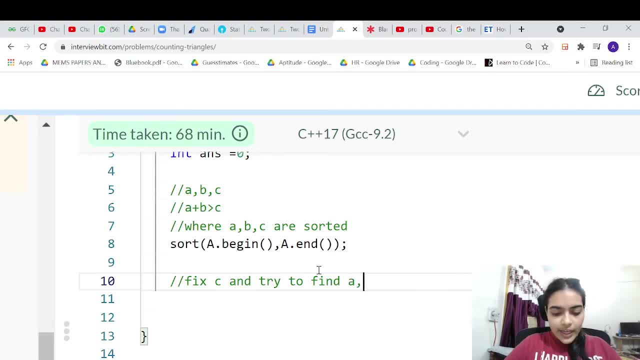 So fix C And try to find Okay A, B that satisfy, A plus B greater than C, Because if C is the largest value we need not even check these two conditions Right. C plus A greater than B, C plus B greater than A- satisfied. 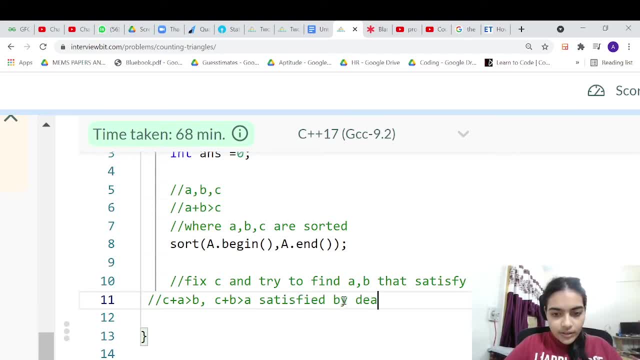 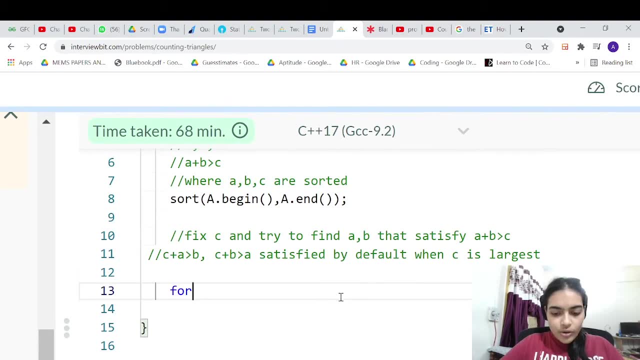 Okay, By default, when C is largest. So this is the concept. Okay, Now let's try to fix C. So for int C equals C, equal to N minus 1.. So we need to declare N, So int N is equal to A dot size. 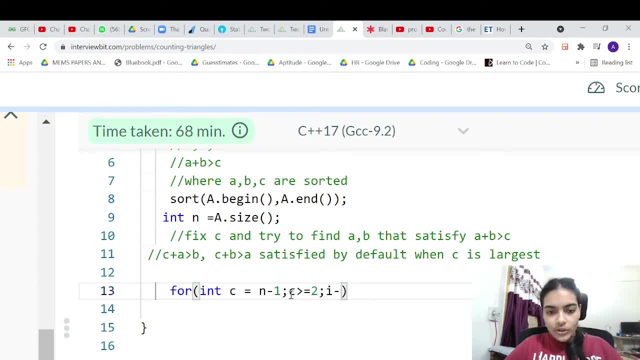 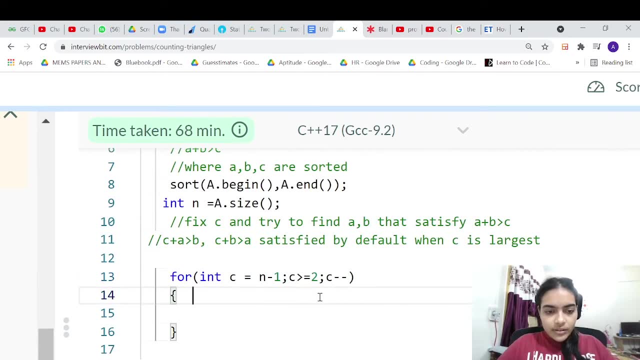 And let me try to fix C. C can go up to 2.. Right, Because you need at least 3 values to form a triangle, And C minus minus. Okay, Now let's try to find A and B, Okay. 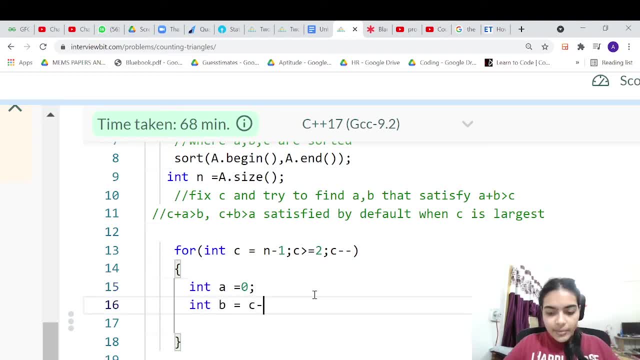 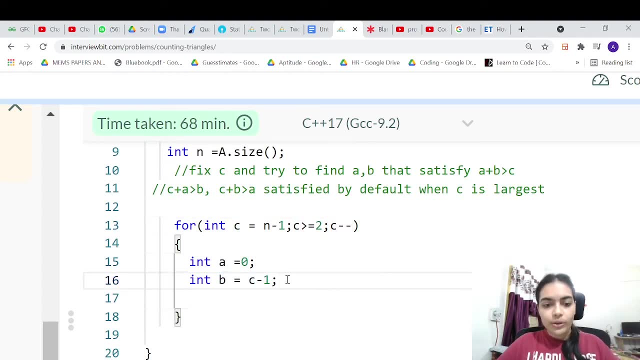 So initially we will start with A equal to 0.. And we will start with B equal to C minus 1.. Right, So Cth index, Ath index and Bth index are the indices that you are trying to fix. Okay, 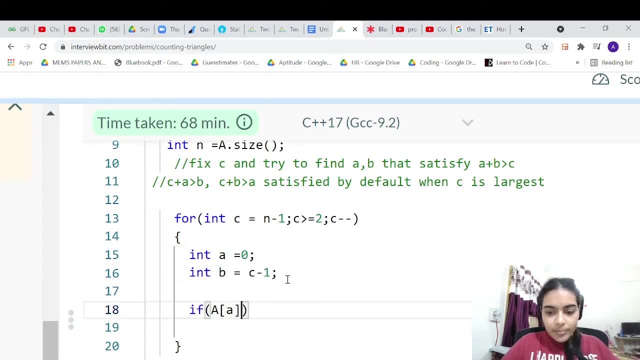 Now you need to check if A of A- Okay- Plus A of B is greater than A of C. This is the condition that you basically need to check. If this is satisfied, then you can move ahead. Right, You can increment your answer variable. 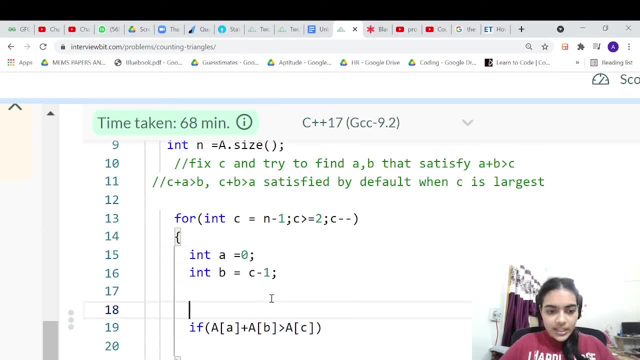 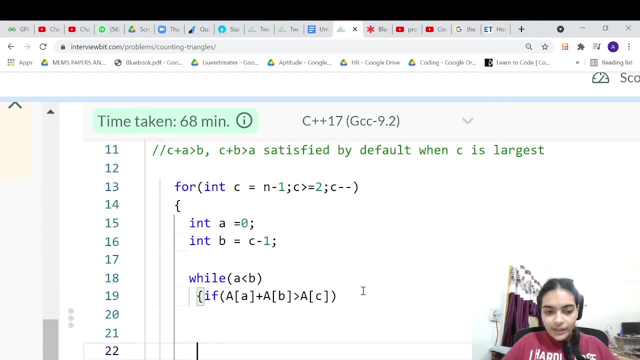 Okay, So this is the condition that you want to check. Where do you want to check this condition While A is less than B? Right, You need to check this. So this is the two-pointer technique that we are using. 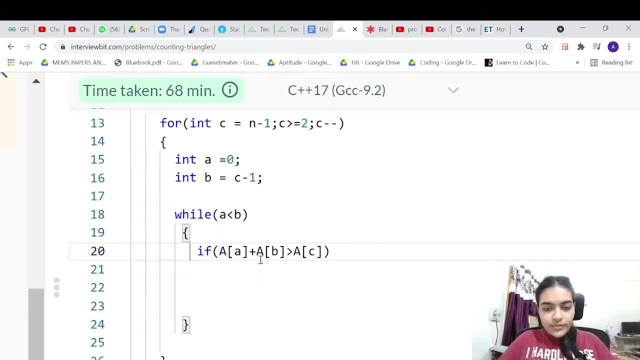 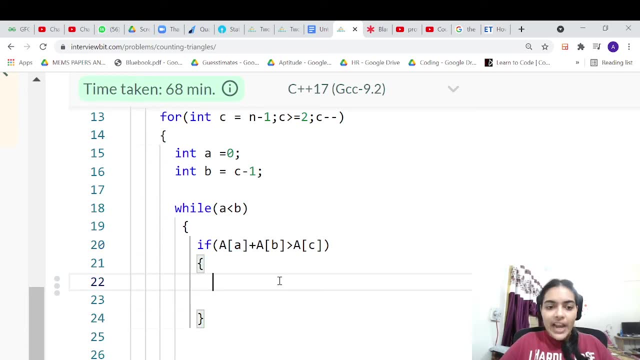 That we just saw in the logic. So if this condition is getting satisfied, What does that mean? All other remaining conditions, All other remaining values of A will be satisfied, As we saw in the logic. So in this case you can add to your answer: variable. 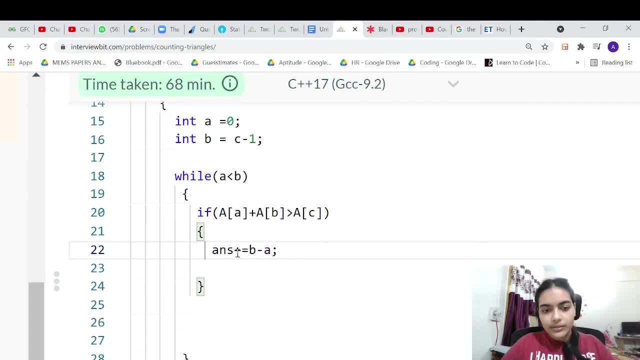 So answer: plus will be equal to B minus A. Okay, All these values will get satisfied. If this condition is satisfied, all other values of A will satisfy. So in this case you need not move your A values and check. 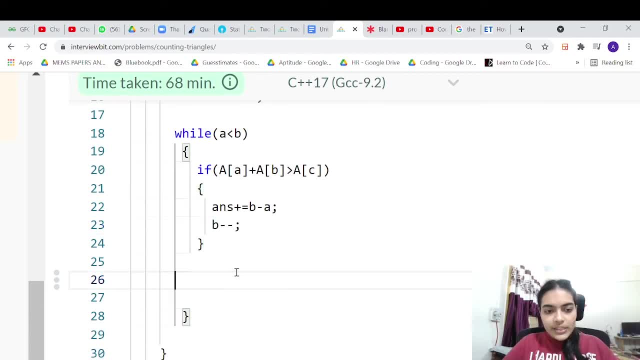 You can move your B value. Right, You can move the B pointer. Else you need to move your A pointer. So see: if the sum is not able to add up and match up so that it is greater than C, You need to try to increase the sum. 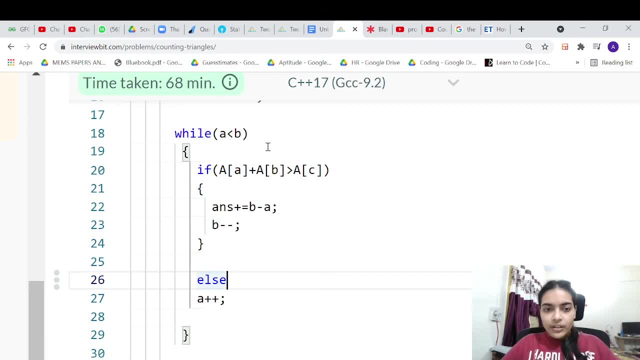 You can increase the sum by moving A, Right. If you increase the sum by moving B, you would have already checked those values or those values will not be existing Right. So you will try to move A and you will try to check the sum.